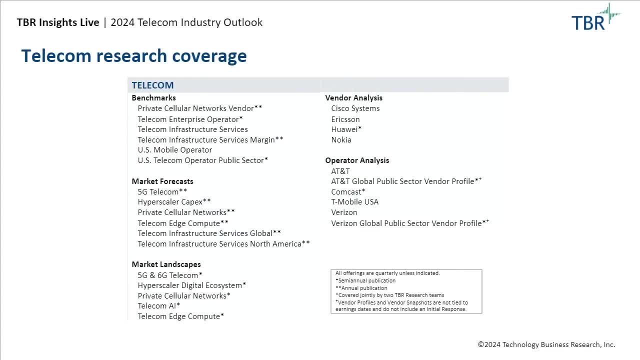 feel free to do so Before we jump into the content. for those of you who aren't already aware, the Telecom Practice has a research portfolio of subscription service And these are the list of the reports that are part of that subscription, And we have a variety of benchmarks. 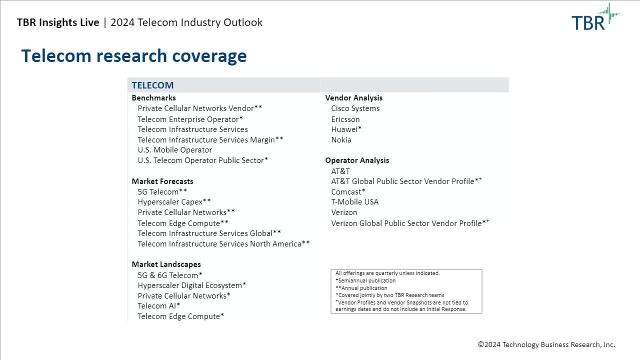 market forecasts and market landscapes that look at key areas of the telecom ecosystem such as 5G, 6G, the hyperscaler, involvement in the industry, edge computing, private networks. We also are launching a new report for this year around telecom AI. We're looking at AI and Gen AI, not just Gen AI, And I want to make that clear. 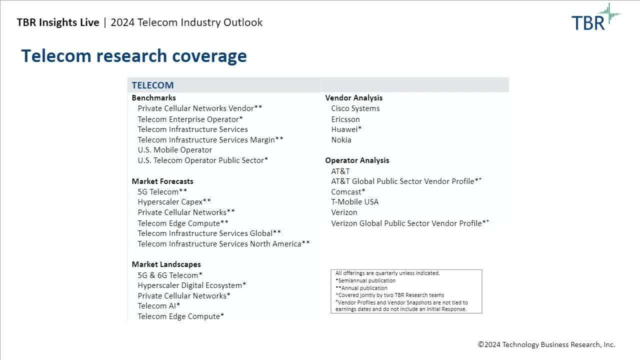 We're looking at the totality of AI as it is coming into the telecom ecosystem in that report And I will be doing a webinar on that In the April-May timeframe. So if you're interested in that, keep an eye out for an invitation. 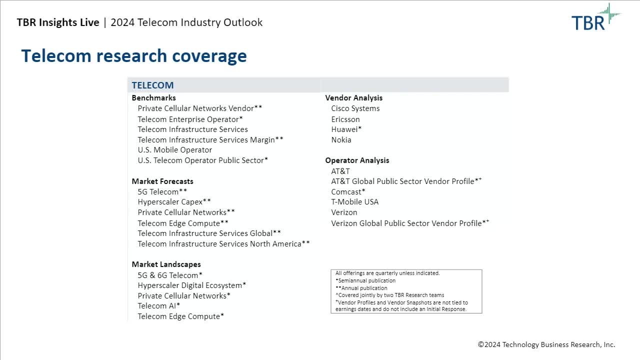 Some of my other colleagues at TBR are also doing AI-related webinars, podcasts, videos and other materials that will be available for general audience viewing. Those will be made available over the next few months and really throughout the year. We have a pretty significant 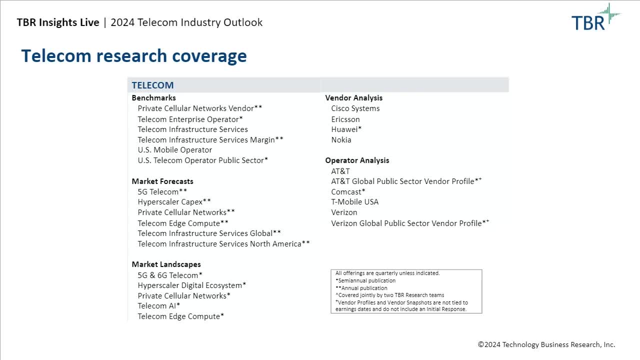 slate of AI-related research coming out, As it pertains not only to telecom but also all of the other major sectors within the ICT ecosystem. We also have reports on vendors and operators. Those are individual reports. We obviously cover many more operators and vendors that are listed there, But those are some of the companies where 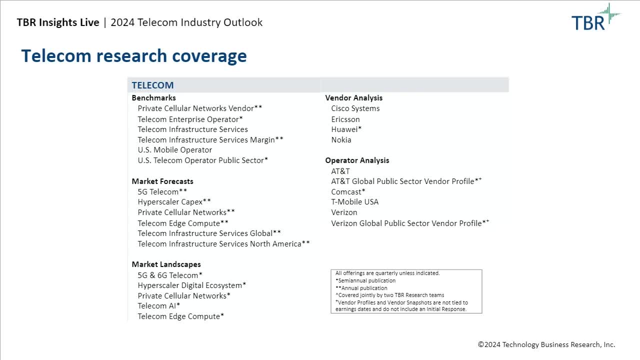 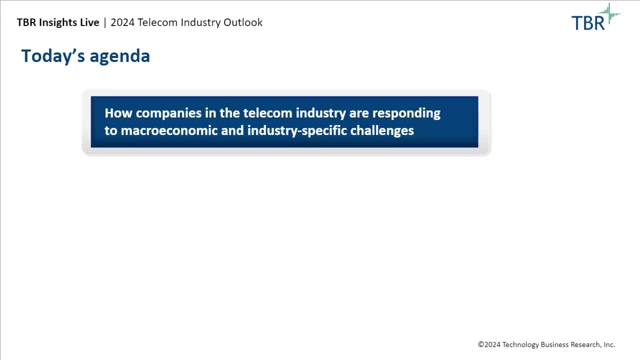 we have dedicated off-the-shelf, if you will, reporting on. So with that we'll go into today's agenda. We're going to be talking about how companies in the telecom industry are responding to the macroeconomic situation. We're also going to talk about industry-specific challenges, So we 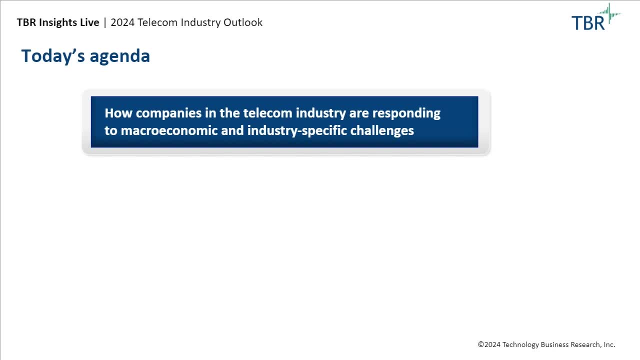 have the macro stuff that's going on- Macro and geopolitical- I'll add that in there- And we also have industry-specific challenges that are coming up and also opportunities. We're also going to be discussing how and why CSPs are prioritizing cash flow management. 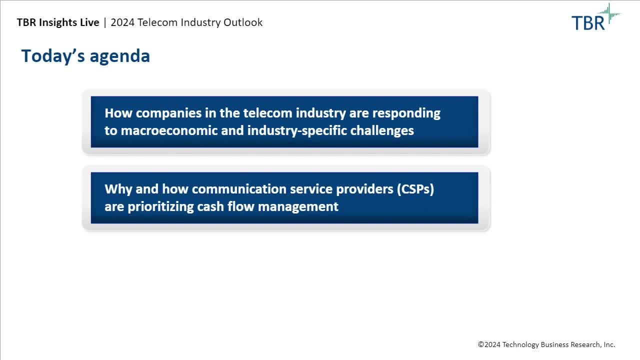 We're going to be talking a lot about cash flow on this call, And you'll see why as we get through the material. And lastly, we will talk about Open RAN. The Open RAN market has not been going well. There's been a lot of challenges with that and we do not believe it's going to be ready. 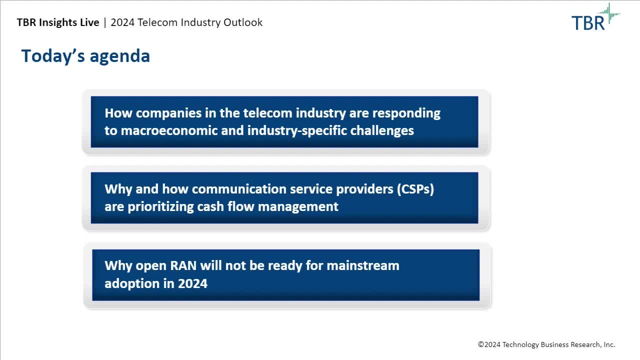 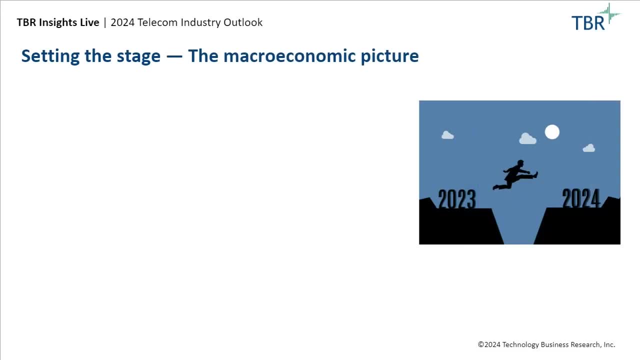 for mainstream adoption this year, And we're going to talk about why that is All right, So let's jump right in. We're going to start with setting the stage. We'll talk about the macroeconomic picture. So there was a variety of challenges and trends that started in late 2022 and through 2023. 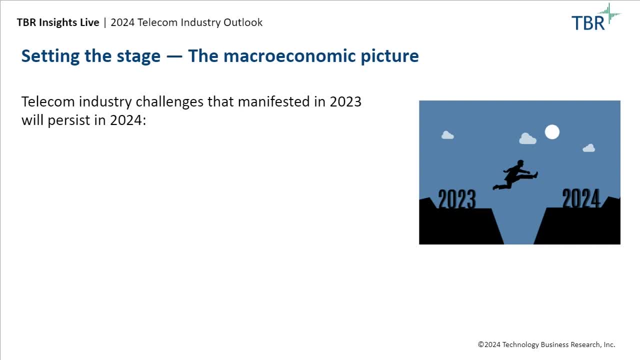 that are going to persist through this year. One of them is inflation. Now inflation rates, generally speaking, have come down from where they were. However, if you look at the long-term rate, if you look at the long guides, that is the long run inflation rate, historical inflation. 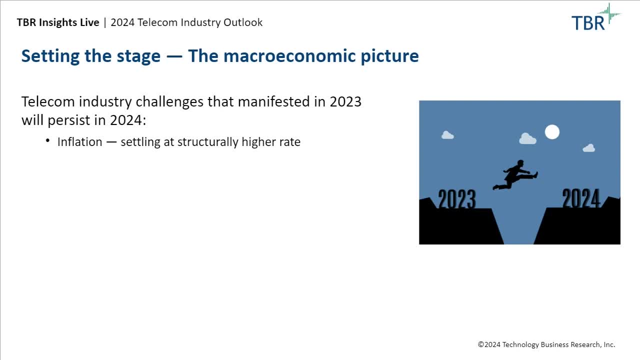 rate and expectations of consumers and businesses for price increases over the future time frame. There is a structurally higher level of inflation now embedded in market psychology, And that means that maybe in the US market, instead of over the last two decades Going forward, we may have 3% or 4% inflation. Now that might not sound. 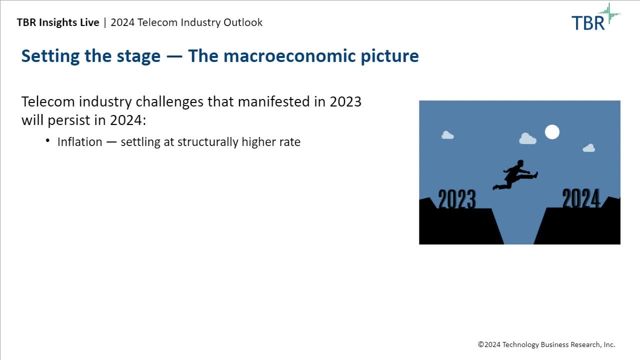 like a big difference, but that actually is a significant change And that impacts cost of capital. Think about interest rates that you would get on debt. It impacts discounted cash flow models that Wall Street uses to ascertain equity valuation. It impacts the prices and the price. 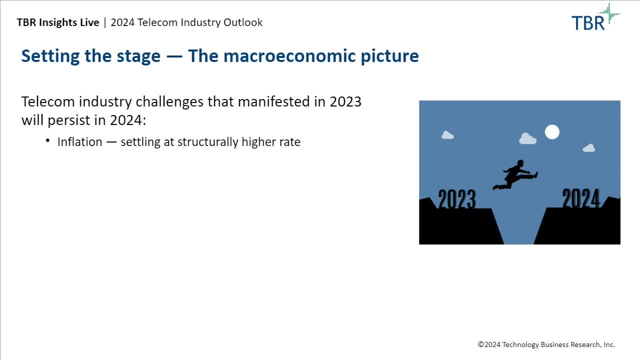 expectations that end customers are expecting. Maybe they have a higher propensity to switch, so maybe we'll see a churn impact. So it might not sound like much, but I want to make sure that I drive home the point that it is structurally higher going forward than what it has been over. 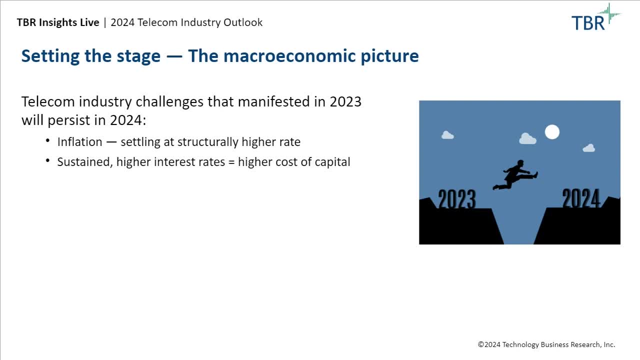 the last decade, One or two decades. The second thing we see- and this relates to inflation- is sustained higher interest rates. Now the Feds, the Federal Reserve and other central banks in other major markets around the world have been doing synchronized interest rate increases over the 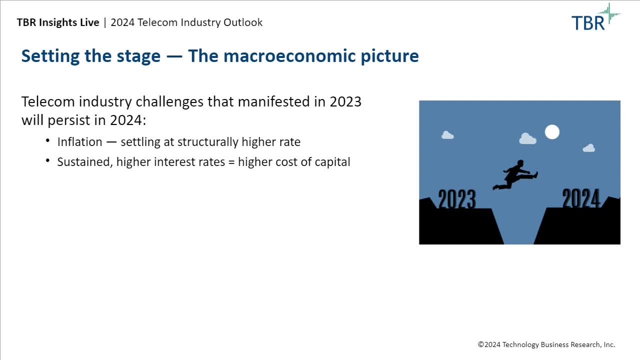 last two years They've kind of flattened out the increases, but we're at a higher level than we were over the last two decades. Now that impacts cost of capital. So when the telcos and the vendors come to market to refinance or 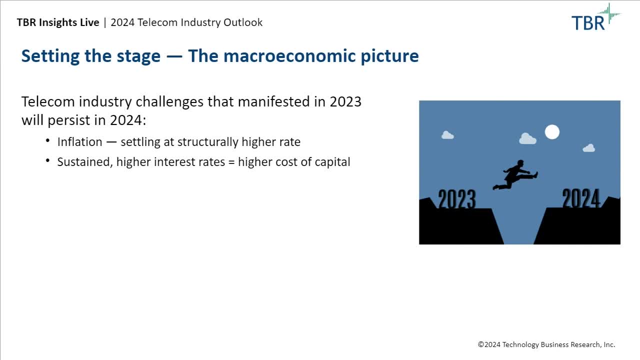 roll over their debt instruments, they're having to pay two, three or more times the interest level that they originally got that debt with. That is very significant and impactful to cash flows. It's impactful to CapEx decision making. It's impactful to how the company's 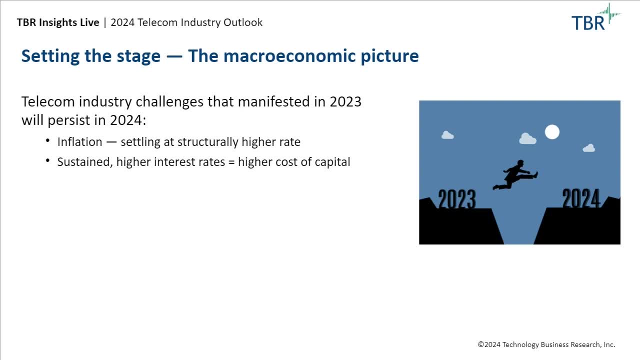 economy can behave will behave to adjust to that new reality. Lack of 5G ROI. So there is one use case that we've seen and we've been looking real hard for this. One use case that's actually driving revenue growth at scale with a positive ROI for the telecom. 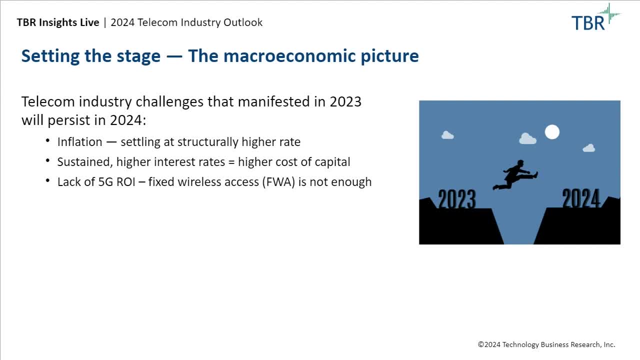 industry globally, and that is FWA. Aside from FWA, yes, there's pockets of revenue growth, but the ROI may not be there or the scale may not be there, And, as we know, telco is a scale business. 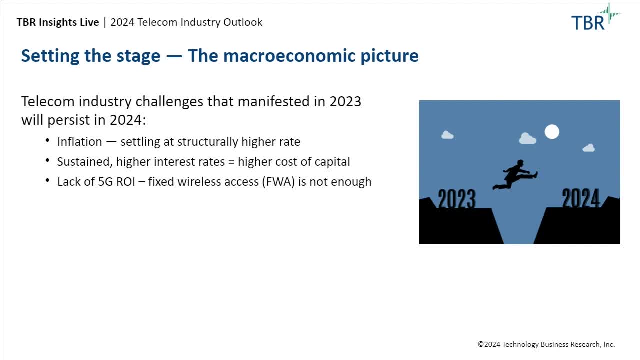 You need to scale profitably, to move the needle on your P&L and to drive earnings growth. The industry is still looking for other sustainable, high growth scalable use cases for 5G, and this is something we'll be looking for at MWC. 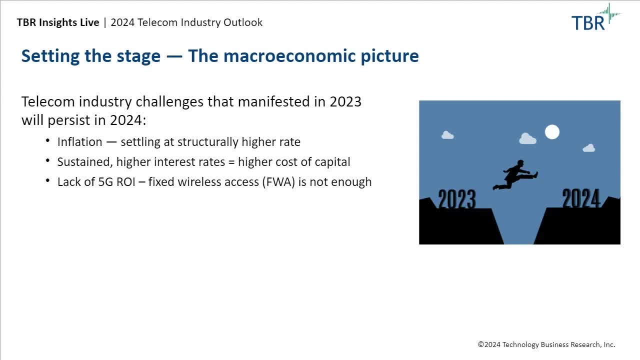 But we don't see any material catalyst on the horizon for this year. We don't see anything aside from FWA. I want to make that very clear Now. after this year, we may start to see new use cases for 5G. 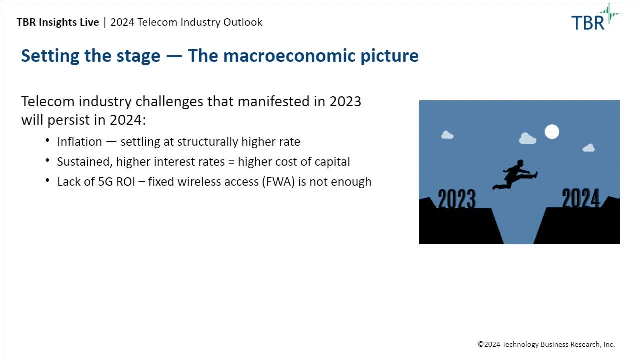 really ramp up and I'm sure we'll be covering that in the 2025 predictions. Technological complexity RAN is problematic. Open RAN is not working out, It's not delivering the outcomes and it's not meeting the expectations, generally speaking. 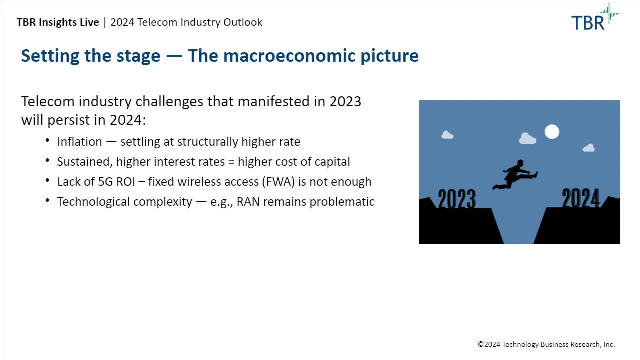 of the telcos. It's falling short And VRAN is doing better than O-RAN. VRAN is more developed than O-RAN. However, doing just VRAN, you don't get the full benefit that the telcos are expecting. 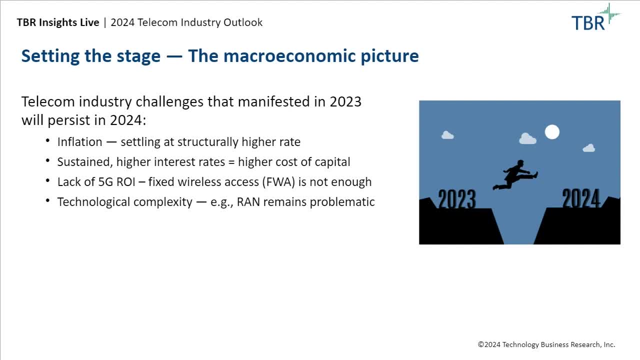 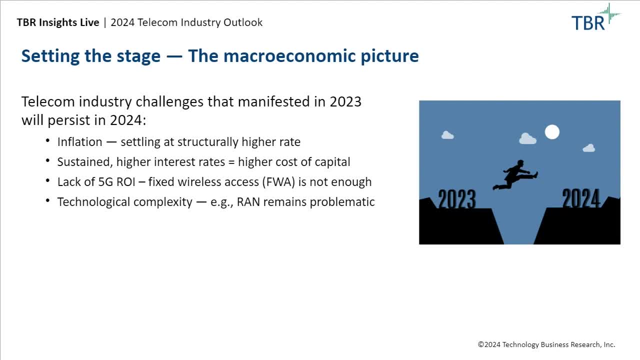 and catalyst moments for Open RAN, But as of for this year, we're not expecting one of those catalysts to happen. We are seeing the end of pandemic-era government stimulus. Now, if you were on prior webinars of mine, we talked about government stimulus during the pandemic era. 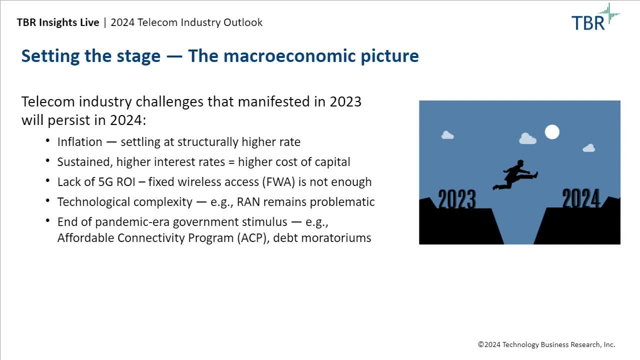 During the pandemic years, governments of the world created, through monetary and fiscal policy measures, over $35 trillion in stimulus. A portion of that went into the technology sector. Around 10% of that, we estimate, went into the technology sector, of which telco is in there. Even 10% of $35 trillion is a lot of money And that money went. 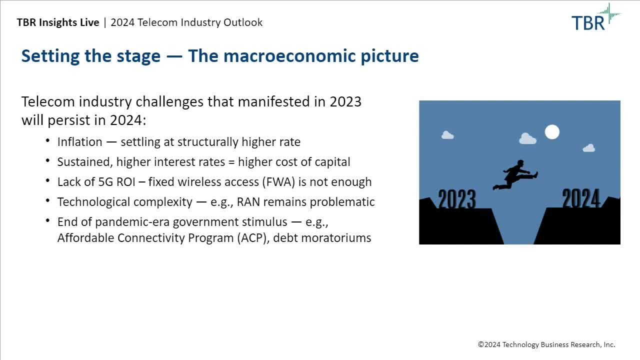 into a whole host of programs: Build America Back Better, the America Recovery Plan, the Tribal Lands Funding, BEAD, the ACP. There were also debt moratoriums, So this is indirect benefit to the telecom industry. People. people's debts were either paid off, such as student loans, 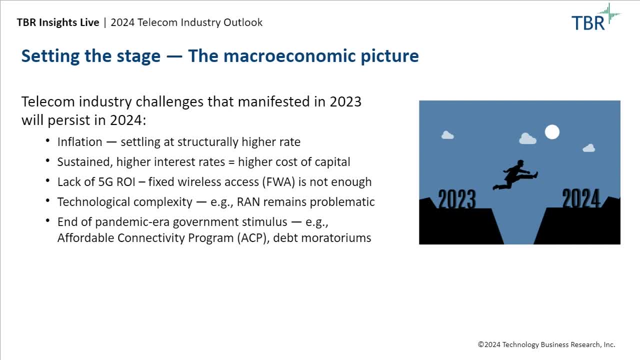 Some of that has been paid off. There were also enhanced unemployment benefits. people were getting Many hundreds- Wow, hundreds- of dollars more per month if they were on unemployment for well over a year. In some cases we were aware of people getting those benefits for up to two years. That is many thousands of 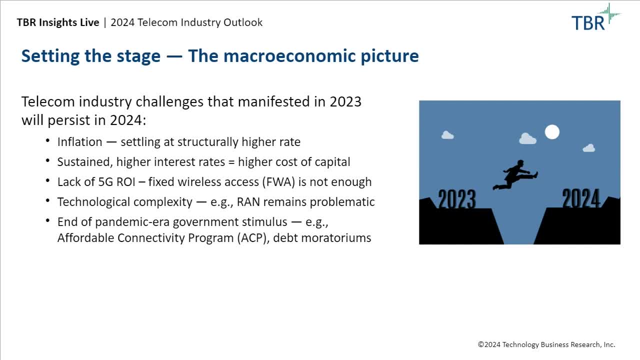 dollars per household. that was a capital infusion. This was not just in the US, this was also in Europe, This was also in some markets in Asia, And when those things happened, people had more money to spend And what we saw was an upswell of device trade-ins. We saw people 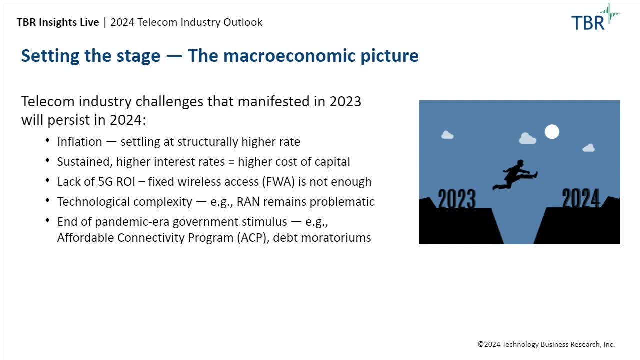 buying new devices- computers, phones, et cetera- for home office use as well as just because they could afford it all of a sudden, And these are things that directly and indirectly supported the US economy, And so we were aware of that, And so we were aware of that, And so 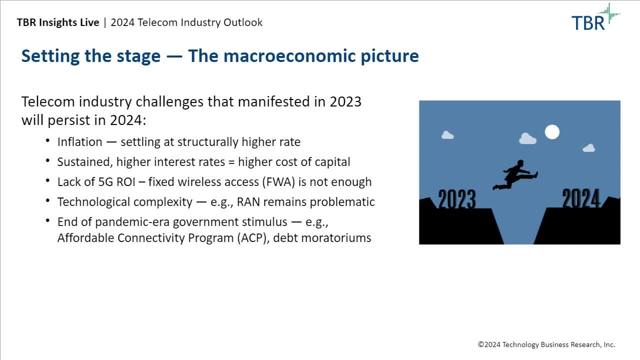 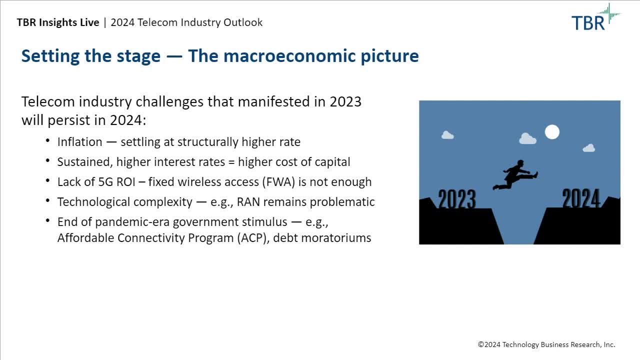 where things have not really ramped up yet, like bead Bead funding is going to happen over the next few years. It started last year but it hasn't really ramped up yet. so those are some of the things to keep in mind. also, some of the swaps, some of the swap. 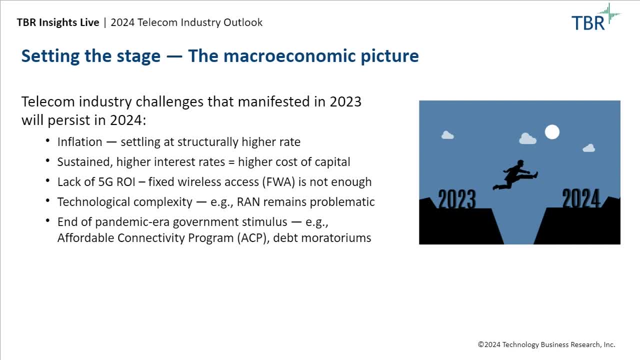 structures in place have not really ramped up yet but generally speaking, if we look at magnitude, the vast majority of that upswell of government supported stimulus is over. so the csps and the vendors have begun adjusting to these headwinds in their industry and in the 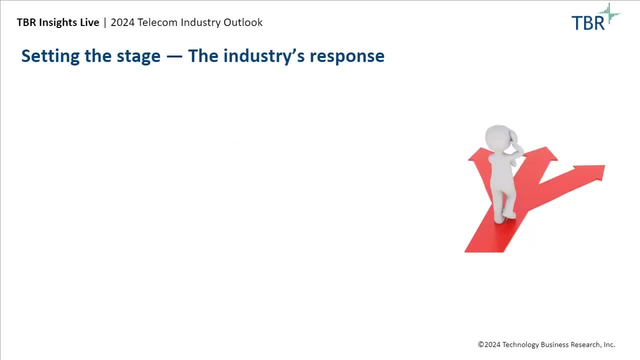 wider economy. now, that's what we're going to talk about going forward here. anybody has questions? feel free to add them to the chat box and the q a box and i'll take them one by one at the end. so what's? the industry's response to this behavior is changing. i want to give you 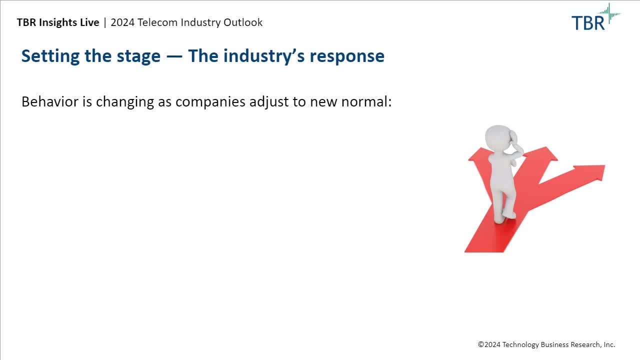 tangible examples of this happening. we are seeing telcos and vendors reassessing their capital structures and their capital allocation and this is leading to a variety of outcomes. we have seen dividend cuts, dividend um completely doing away with the dividend. we've seen capex reduction, not just because they've done nationwide. 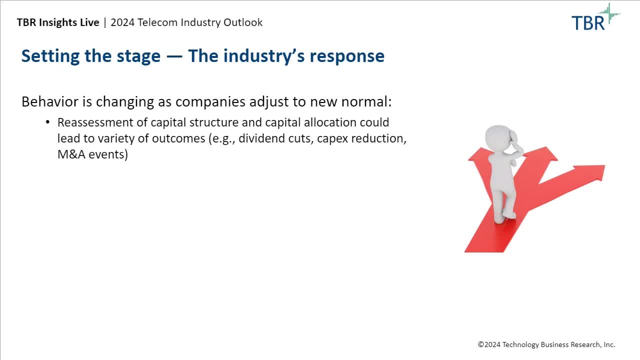 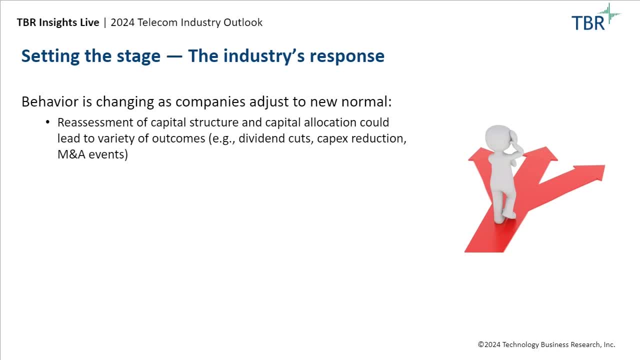 significant increase in m&a. we are seeing write downs, um and asset revaluations in the us market. there was a tier one, telco- i'm not going to name the name, but they wound up writing down over five billion dollars of. they took an impairment and they took an impairment, and they took an impairment. 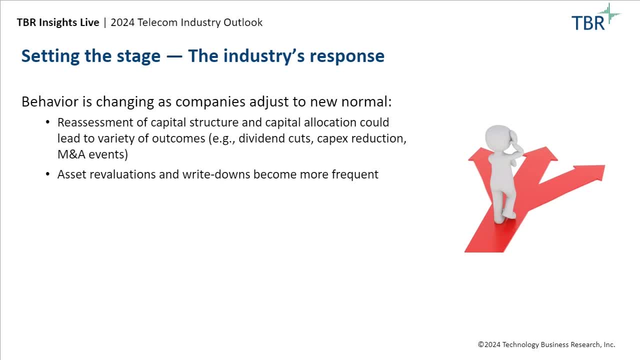 for their enterprise business. now there are. that is just one example. we have seen many asset write downs at various telcos around the world over the last 12 months. we are expecting to see further asset write downs. these are one-time hits to the balance sheet. they're usually non-cash in nature. 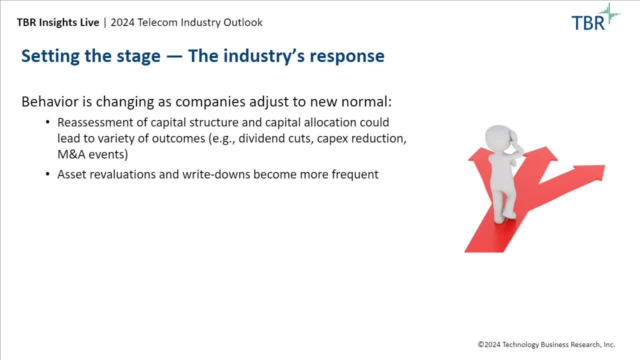 but they are telling of what is the real value of the assets the telcos are carrying, what is the value of their brand, and those are things that are very interesting to consider in the context of outlook. we have seen several operators scale back their fiber build targets. 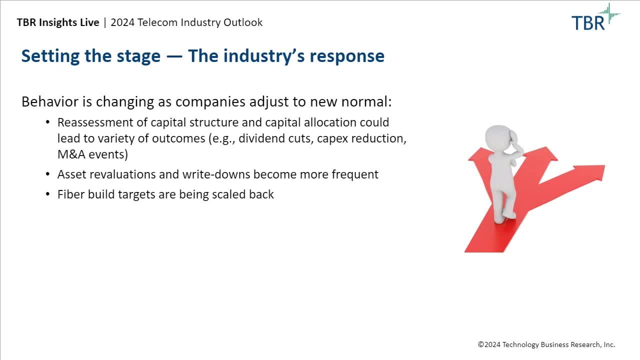 i'm not going to name names, but there were, uh, two or three telcos in the us market. i think there were three that are have officially stated that they're doing this. um, that they are, so maybe they were planning to do. x million homes passed with ftp. what we have seen. 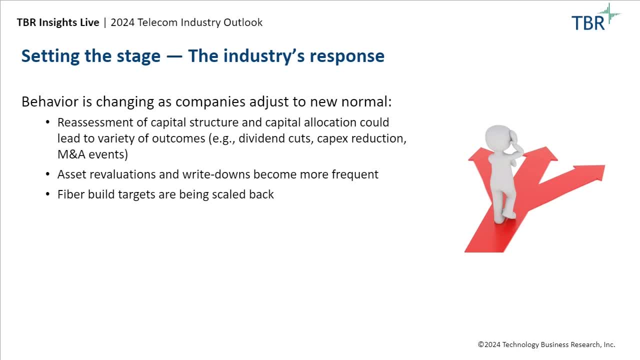 in the last 12 months or so is that they have reduced the scope of what they're going to do for a bill. there's various reasons why they're doing that, but one of the biggest reasons why they're doing this is because the cost of capital is fundamentally higher than when they originally. 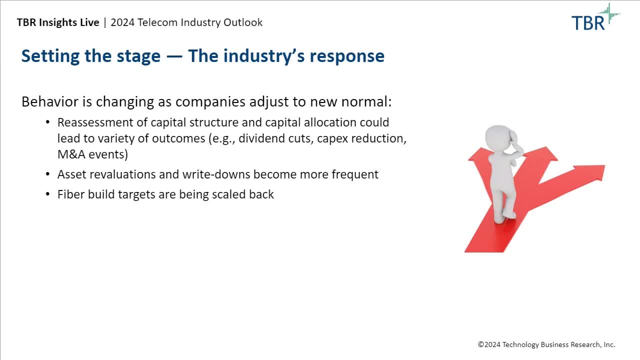 put those build targets out, and what that means is that it is going to be a lot more expensive, and it is going to be a lot more expensive than what they originally wanted to do, and it is no longer roi positive for them to do the full scope of what they originally wanted to do. that is a significant 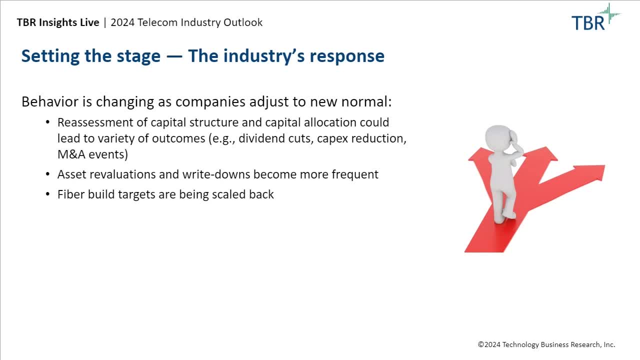 development. okay, these are examples of behavioral changes among the telcos and among the vendors. capex budgets are being reduced in many cases. we have seen very few telcos globally when we look at the global landscape: very few instances where telcos are guiding to higher capex standards. 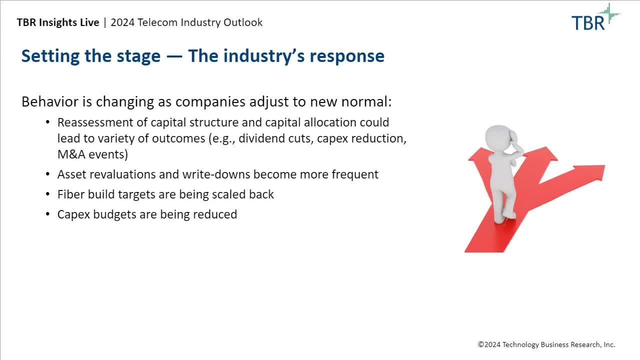 this year. very few examples. the vast majority of telcos that are putting out guidance are indicating either flat capex or lower capex for this year. so this comes back to the cfo and one of our one of the things that we will be watching very closely, this year especially, is more examples of behavioral changes and these things are going to 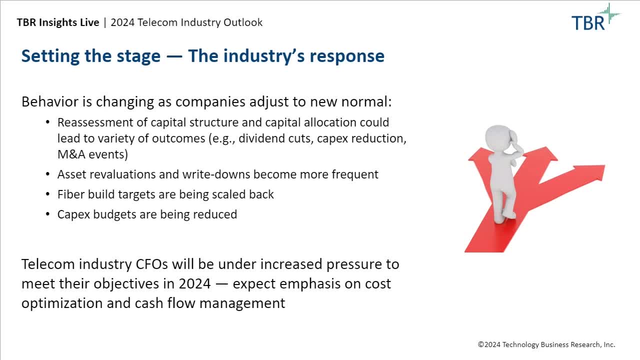 come from the cfo uh department and when you see these things, you will know that these are adjustments to the new reality, the post-pandemic economy, the non-stimulated, artificially supported economy. um, so everybody's adjusting. now to what is that new level going to look like? 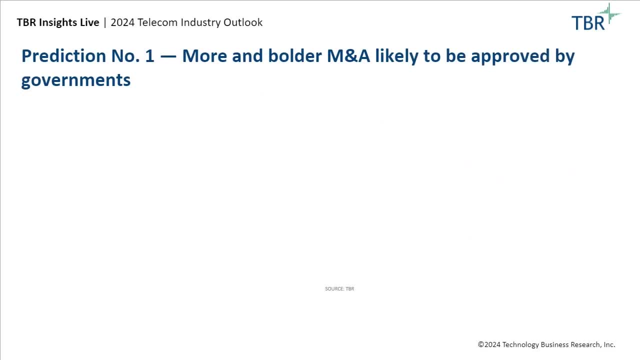 okay, so this brings us to the first prediction, and i mentioned it before. but m a? um, the m? a market was relatively subdued the last two years, relatively subdued for tel, for the telecom industry. um, we are expecting this year that we are going to see a significant increase in m a. 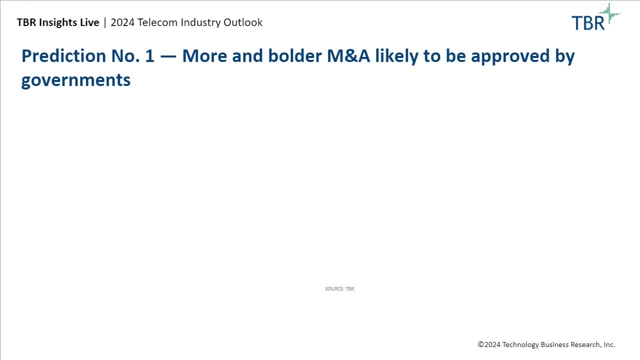 um, some of it will be uh forced and some of it will be actually reduced, and some of it will be more uh, uh reduced, uh two years later, as we look at the digital world as well, but this is a lot of time of it will be pre-planned Now. when I say forced, what I mean by that is, we will see situations. 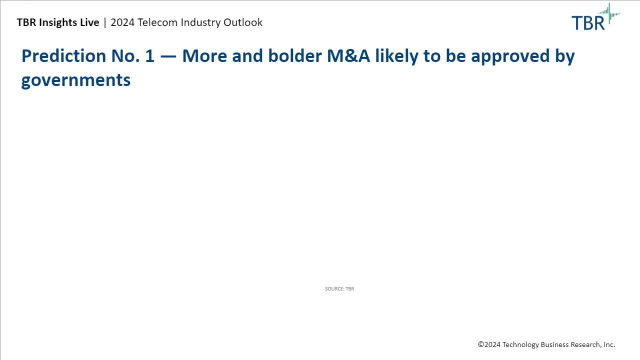 where operators and vendors get into a financial- they have a financial reckoning, let's put it that way- where they need either a massive capital infusion to continue their business, they need to do a structural sell-off of assets to pay off debt, they need to make structural changes. 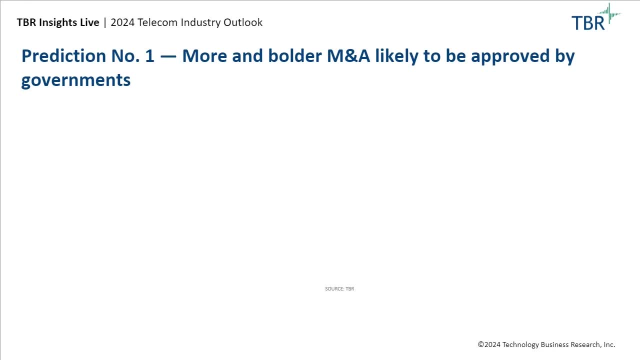 because the business structure that they have is not aligned with the post-pandemic economy. I'm going to give you guys examples of these things. I'm not going to just say, like I'm not going to say these big statements without giving examples. I'm going to give examples for everything. 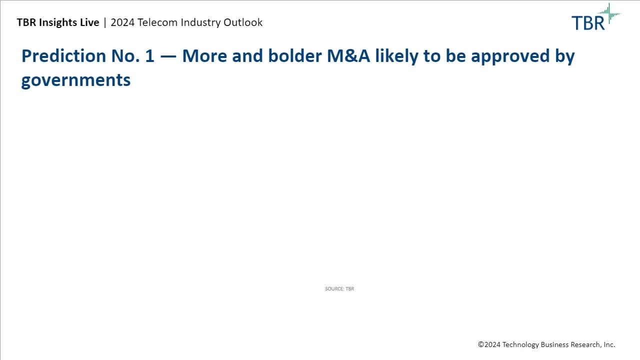 that we're showing here. So and then pre-planned M&A would be situations where you have a telco that or a vendor that is in a relatively strong financial situation to take advantage of market opportunities that arise from other entities that are struggling, or 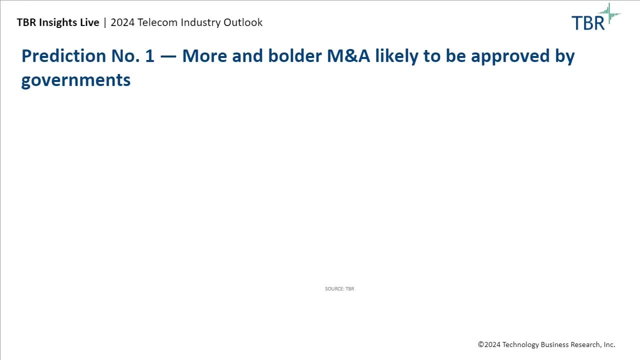 where the valuations are coming back down. Maybe there's a software company or a cyber company or a services company or another telco whose valuation was very high. maybe it gets revalued and maybe all of a sudden, the ROI and the deal sense the deal all of a sudden. 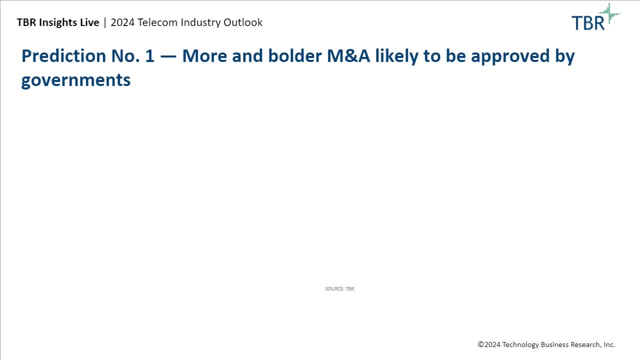 makes sense. We're going to see situations of this. We also expect that these things are going to be approved by governments. So historically there's been resistance to doing fewer than three tier ones in a market. We are starting to see two tier ones in a market and that's starting to become 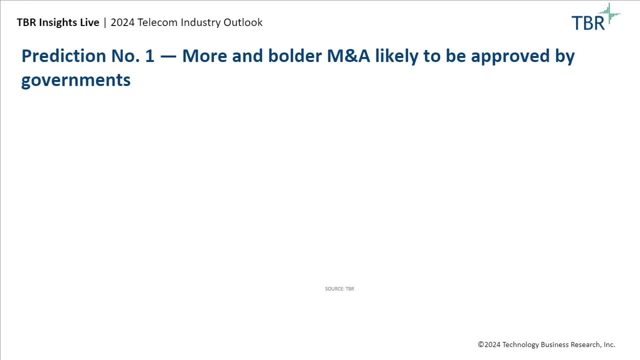 where things may be going, Not in all markets, but in select markets. we may start to see even further reduction of tier ones in a particular market. I'm going to give you guys examples of these things, so just hold tight. So 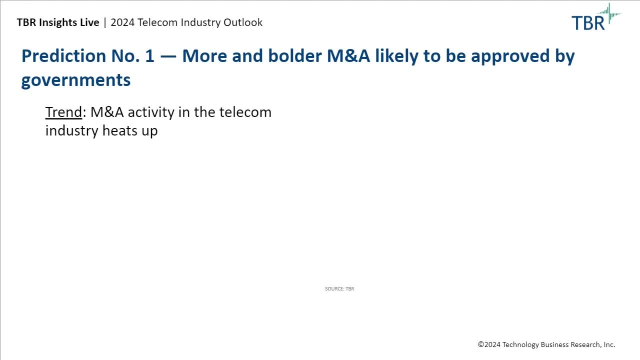 the trend is that M&A is going to heat up this year. We are expecting to see a lot of stock deals where, because the cost of capital has increased, we may see more equity components to M&A than cash components. That's something we're going to be watching. That's what we're expecting. 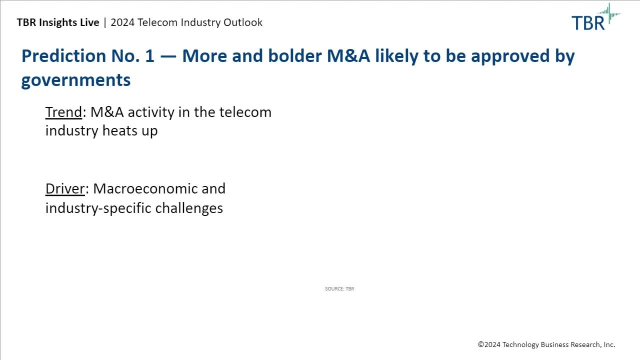 The driver of this trend is macroeconomic and industry-specific challenges, which we've already discussed. what those are? some of them And the result? we're going to see fewer but larger and stronger entities remaining on the vendor side and on the operator side. 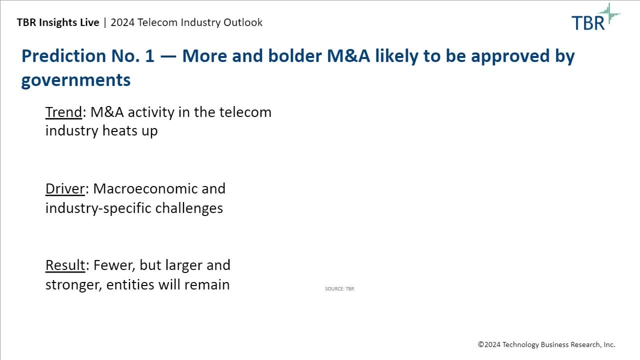 And when I say operator, I'm including telcos, fixed and wireless, I'm talking about the satellite connectivity providers and I'm talking about the cable codes, That's. when I say CSP, I'm including all of those entities in that bucket. 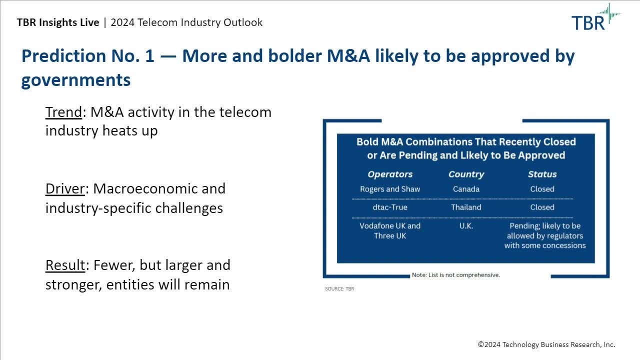 Okay, so examples. So there have been bold M&A combinations that have already happened in the recent past, and these are things that maybe five or more years ago the governments would not have allowed to happen, but now they have happened, And the Roger Shaw deal is one of those situations, Again, five or more years ago. 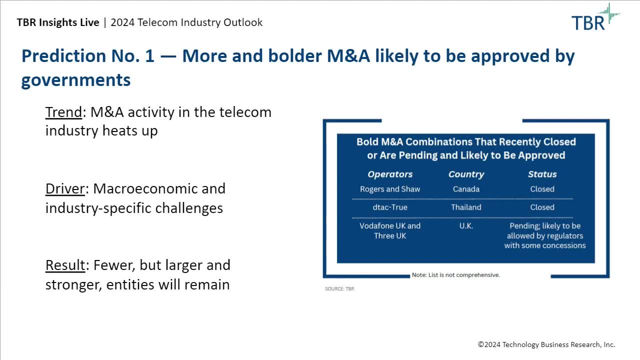 before the pandemic, if Rogers approached Shaw and said: we want to buy, you guys and the government's going to get this, this is going to be approved, it wouldn't have happened. It would have been a flat out. no, no matter what. no concessions are going to make this happen. 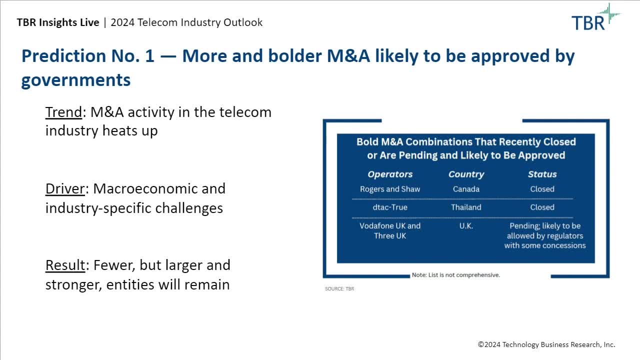 Okay, that was the environment at that point for that type of an acquisition right, Where the number four player is being taken out by the number one player. That deal has since closed. There were concessions made, of course, which is to be expected. Videotron did take a portion of. 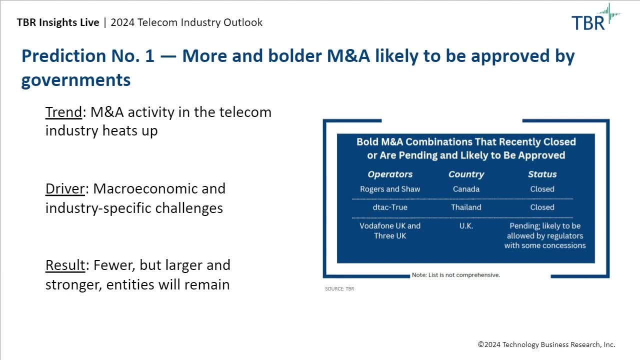 Shaw to balance out the competitive landscape post acquisition. but the point I want to stress is that deal was ultimately approved. The DTAC True deal in Thailand also closed. That would not have happened pre-pandemic. These are situations where the deals all of a sudden. 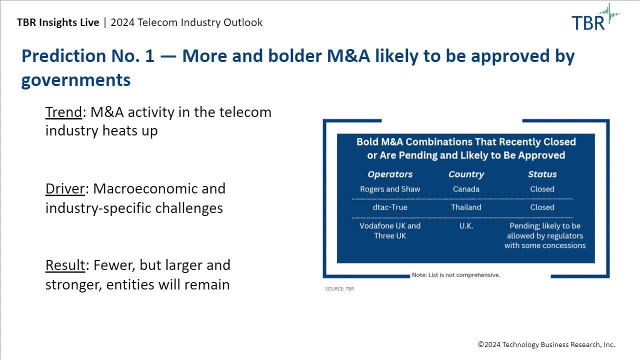 they're being green-lighted with concessions, of course, but they're being green-lighted. One that's in play right now, which we expect will happen, is Vodafone UK and 3UK. We do believe this deal will happen in some way. There will likely be concessions, but the deal will get approved. 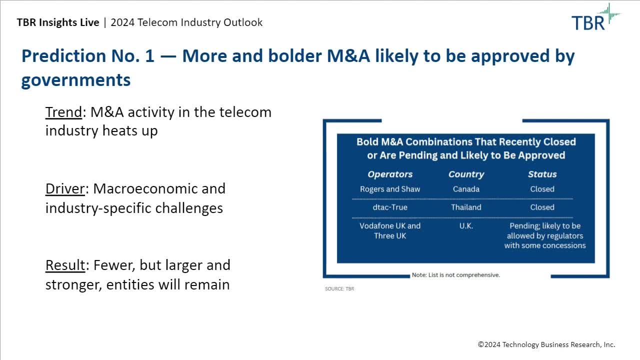 That is what we believe is going to happen with that deal. We are expecting at least a few more big M&A events to happen this year in the telecom industry in various parts of the world. The stage is set for this to happen. The trends are in place to 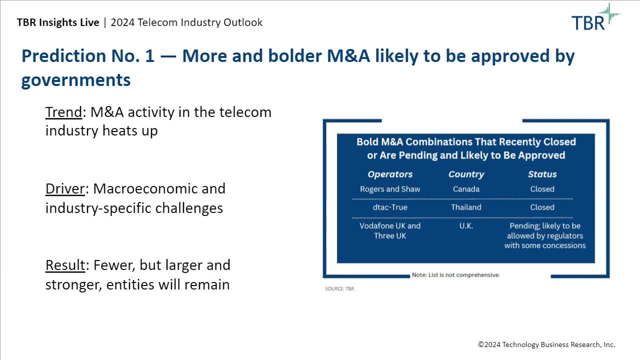 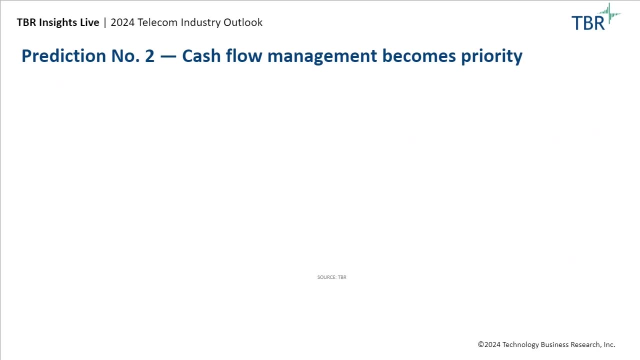 move the industry in this direction, and the government regulatory environment and the competitive landscape is such that we think more deals are going to actually get green-lighted. Okay, so the next prediction it is cash flow management. Cost of capital is increasing and this is driven by central banks. 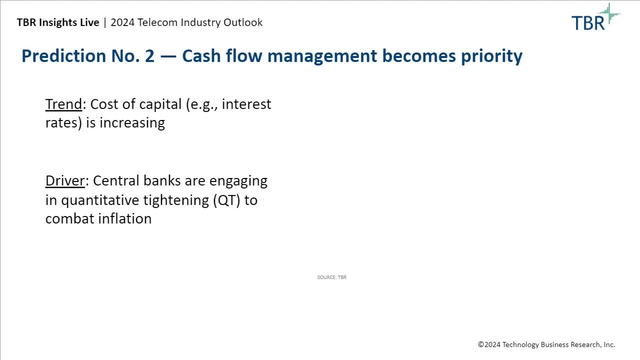 engaging in what we call quantitative tightening Now, post great financial crisis in 2008,, 2009,. what the central bankers of the world did is they reduced interest rates to artificially suppressed rates, dropping them to levels never seen in the history of. 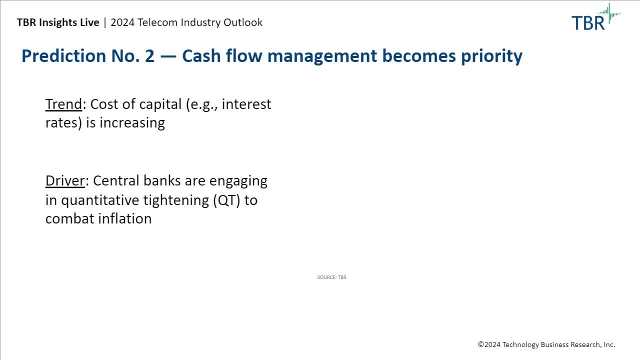 mankind. okay to zero. in many cases, zero interest rate, and there was even negative interest rates in Europe. In many countries in Europe they had negative interest rates. That is historically unprecedented. Nothing like that has ever been seen before. That is what QE looked like. The reason the governments did that was to 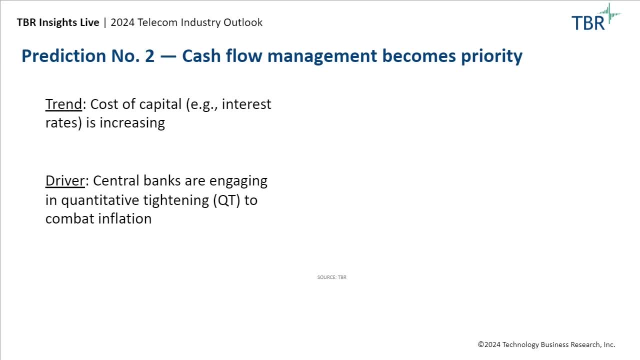 support the financial system and support the economy. through that tumultuous time. It did wind up working, thankfully. However, it created a moral hazard situation and it created a situation where governments became accustomed with sticking with QE because it was driving their economies at a higher rate of growth than what they were getting. 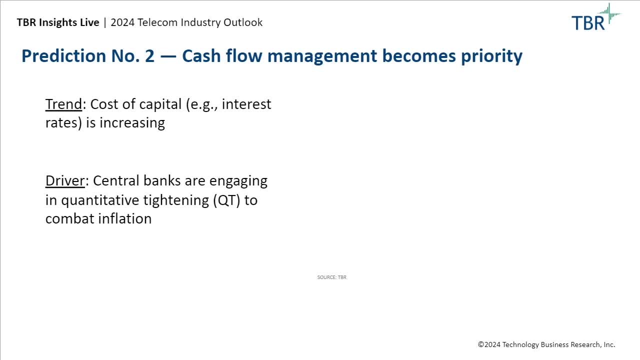 beforehand. When you reduce the cost of capital, you encourage investment, you encourage spending, and that's exactly what we've seen. We've seen those things happen not only in the telecom industry, but in the entire world, So we are expecting now that things are moving away from QE. there's still elements of QE in. 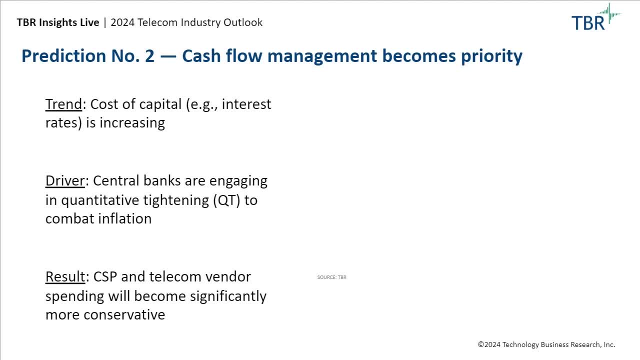 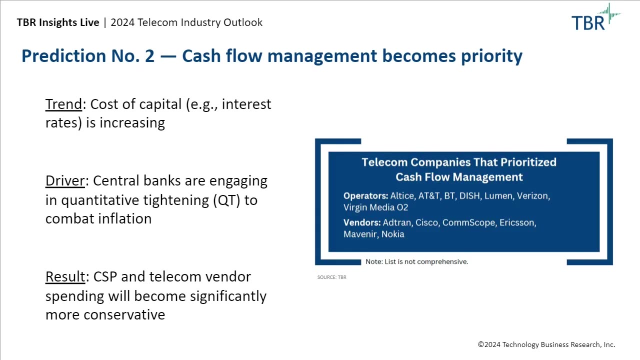 place. but now that there is a pivot away from QE towards QT, we are expecting to see telecom entities becoming more conservative with spending, And I want to give examples of this. So the list of names here are companies that have explicitly said on earnings calls at investor. 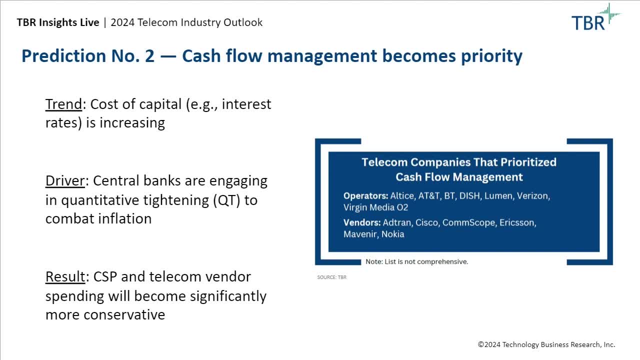 presentations, in interviews on business media, that they are focused on cash flow, And this is a trend. Since we made this chart in November, we've seen several more companies to be added to this list, So this is definitely a trend. The amount of times that the word cash 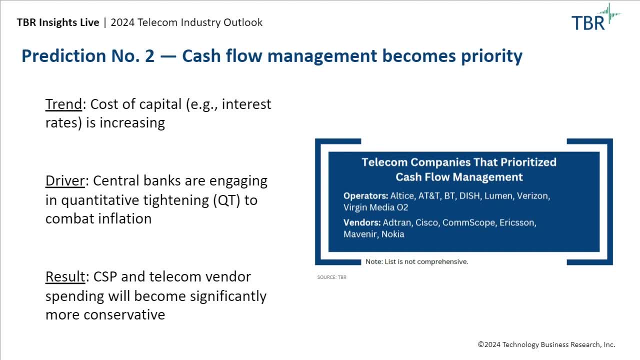 flow or cash is being talked about on earnings transcripts in the telecom industry has significantly increased over the last two quarters. I would say We've ran an analysis. we have an AI. I think that we ran the transcripts through in the industry to look at number of times of mention. 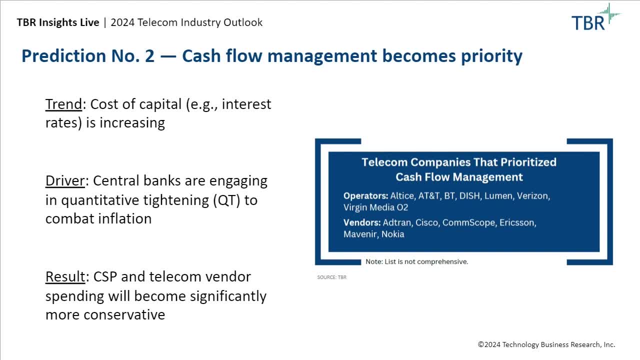 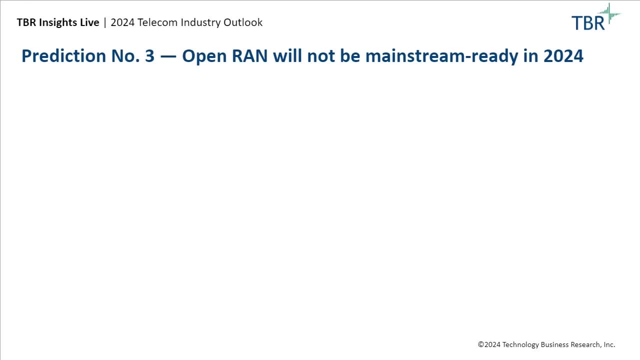 and we do see an upward correlation there in companies- are talking about this much more. Okay, The third prediction is about Open RAN. Now, Open RAN was. everybody was talking about this. you know, two years or so ago This was going to revolutionize radio. I ultimately believe it will. 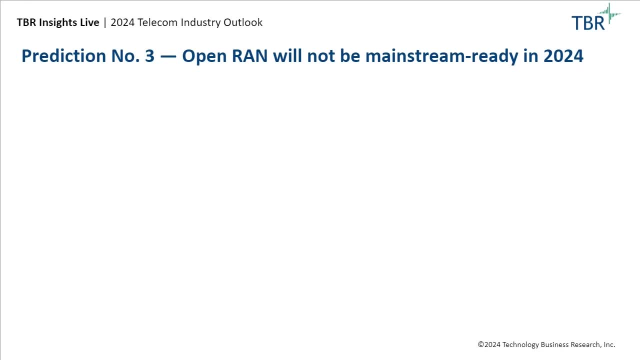 This will happen. The question is, when is it going to happen? What has wound up happening is the complexity and the vested interests. the power of vested interests in the ecosystem have been insurmountable challenges thus far, And what I mean by that is companies that may. 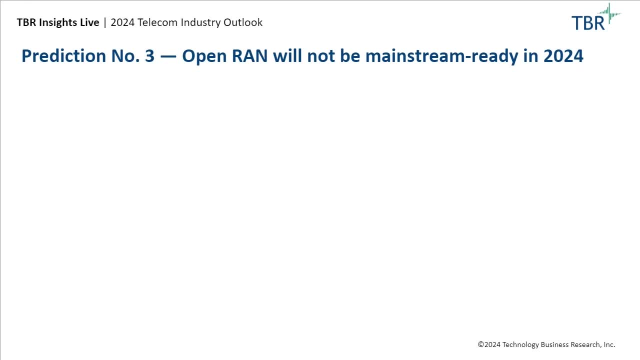 not want to open their interfaces because there's a competitive aspect to that. They may have value at risk by taking that strategy. So they didn't participate. There is embedded install base in the ecosystem in networks globally where introducing open rent into brownfield environments is extremely expensive. 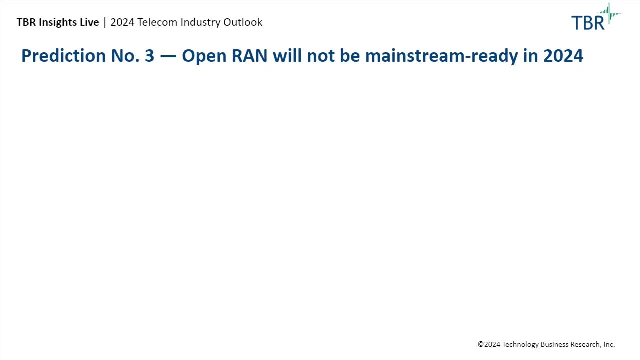 And there's challenges with feature parity, backward compatibility, seamlessness of service. These are challenges that have proven to be extremely expensive and it has significantly slowed the momentum of open rent. Virtual rent is doing relatively better. However, we do still need silicon innovation because hardware acceleration is required. 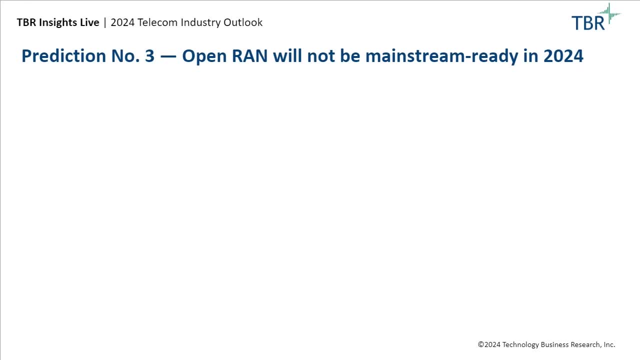 still for VRAN and that is very power hungry and it doesn't run efficiently. There are companies working on silicon. It's very difficult for silicon to run radio workloads much, much more efficiently at the edge of the network Once those types of chips start coming into the market and getting into commercial equipment. 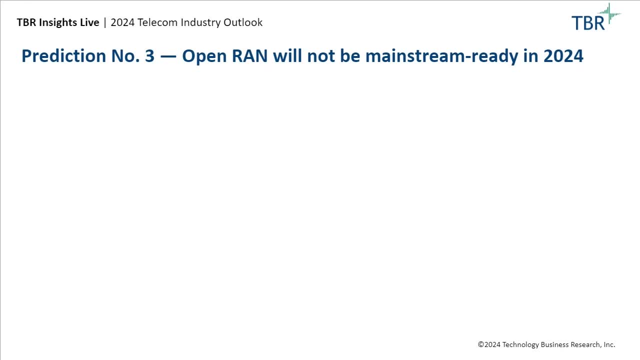 we're going to start to see real benefits coming from virtual rent. There are other benefits of virtual rent that are being realized today, such as composability of software, software chaining, things like that- service chaining. So there's good momentum. There's good momentum already for VRAN, but from an open rent standpoint it's going to 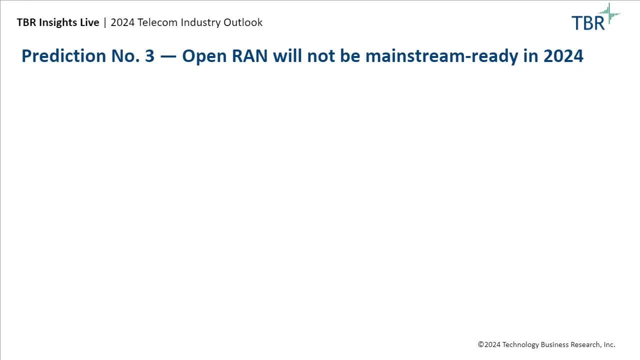 take some more time for that to build momentum again, and it's not going to be this year. So again, the complexity is slowing this market down quite significantly. Classic RAN is going to stick around for quite some time, at least through this decade. 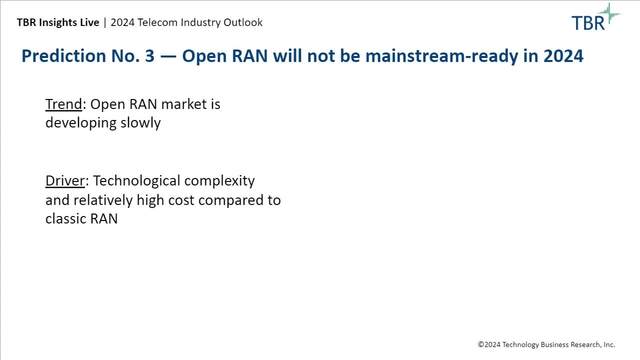 Classic RAN is going to be the de facto architecture And the result is, as we said, open RAN is going to – we don't see a catalyst moment for open RAN this year. if I put it another way, That's how I would describe it. 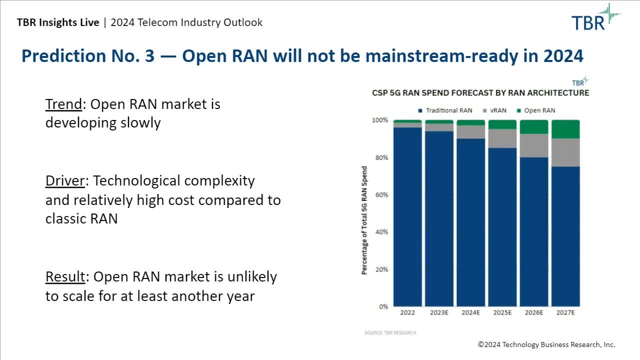 So what we have here is a chart with some data that we've generated. This looks at the three radio architectures. So you have the classic or traditional RAN, you have VRAN and you have open RAN. Now, ultimately, the end state radio architecture is going to be the one that's going to be the 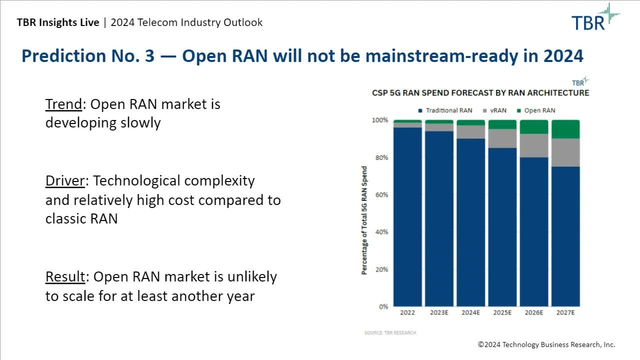 one that is supposed to shift to open virtual RAN both. It needs to be open and virtual. That is the end state of radio architecture. But what we're seeing is operators are starting – in most cases they're starting with one or the other. 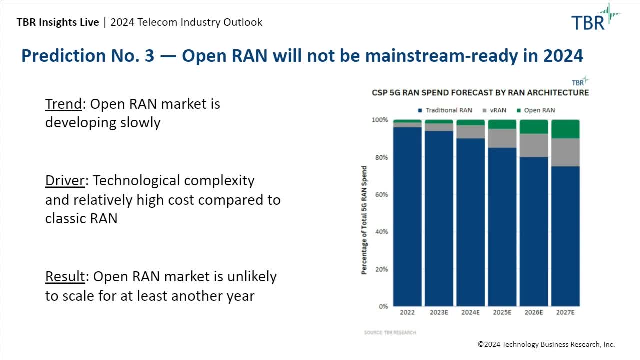 In most cases, that's what we're seeing. So, as you can see here, we project out five years out to 2027.. The vast majority of the radio market in – later this decade is still going to be classic RAN, with VRAN and O-RAN growing in the mix over time. 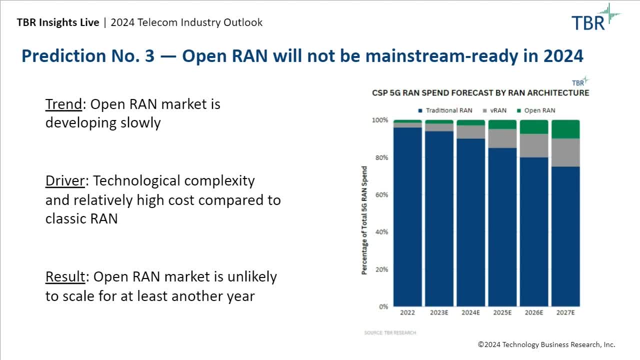 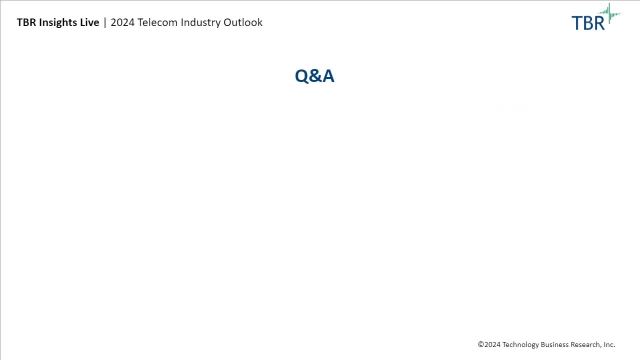 with virtual RAN growing at a faster rate compared to open RAN. Okay, So that's the three predictions And with that we'll open it up for Q&A. I see there is some questions in the queue, so I'm going to start and work my way up. 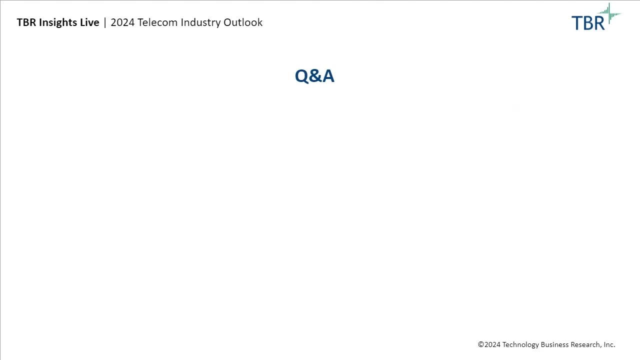 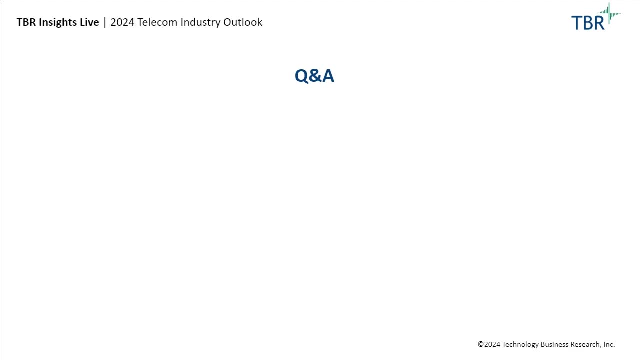 and that the number of cuts that the market is expecting, which is five to six this year- that's what wall street is, that's what the general consensus is in wall street- is for five to six interest rate reductions this year, which, by the way, is historically like unprecedented amount of reductions. um, so he's indicating to maybe two or three reductions. 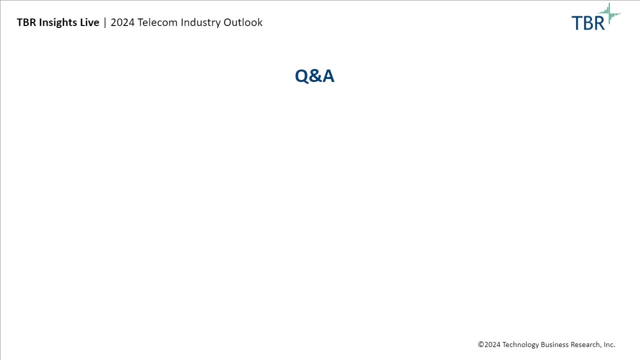 okay. so he's setting expectations and calibrating market expectations with the economy, and so i would say, yes, it's true that rates are probably peaking. there is some geopolitical issues in the middle east, in asia, that could create a supply chain that could create a supply chain that could. create a supply chain problem, could create an energy crisis. that could restart interest rate- higher interest, higher inflation- which would cause the central bankers to either keep the rates where they are or maybe even increase them again. but barring something like that happening, let's say the rates come down two or three cuts this year, 25 basis point cuts. so in the states, you go from a five to six basis point cut to a five to six basis point cut, and then you go from a five to five and a quarter percent down to say four and a half percent. um, the telcos are still paying two, at least two times the interest rate at those levels than they were just, you know, 18 to. 24 months ago. so on a relative basis, yeah, it's. it's a little bit better. a little bit better, but it's still significantly higher than what the industry was accustomed to, uh, for for a long period of time. so i would like to. so i think my, my short answer to that is yes, that's, that's probably true. how? 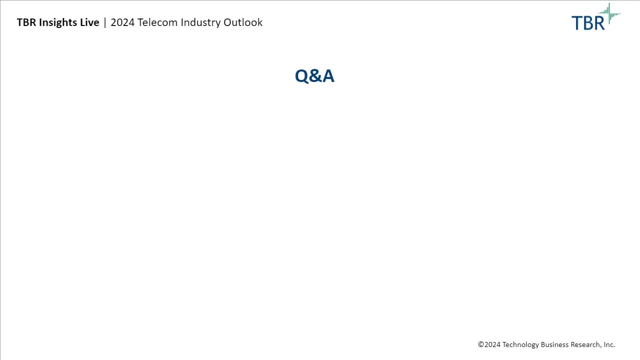 you're framing it um, but you have to look at it in terms of relative um changes over a time period and how much things have changed in an absolute way from one time period to another time period. okay, so the next question is: does the success of 5g and fwa reduce the impact of the reductions of fiber build-outs? i think it does. um. that's definitely a driver um, but i think so when we did an assessment of the the several companies that have announced a scale back in the in the fiber builds. there are several reasons driving that. we believe that one of the biggest reasons is cost of capital, because your marginal homes passed or businesses passed all of a sudden, because the interest rates are higher than the higher it all of a sudden. the roi doesn't make sense, so they would. they would say, okay, well. 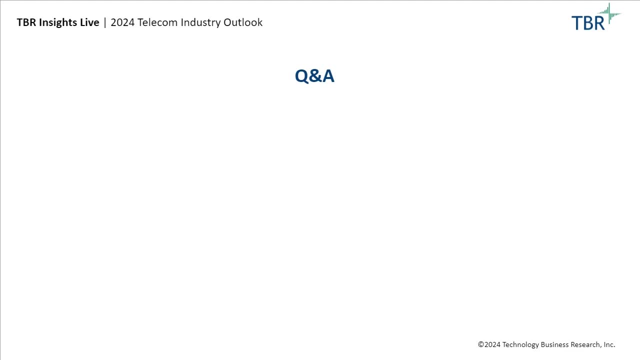 we're not going to do these markets now or these neighborhoods or whatnot, because it it the the numbers don't work anymore. when they run the numbers, they don't, they don't look as good as when they ran them originally for the target. so i so, i, i so, yes, fwa, i think, does impact that that. 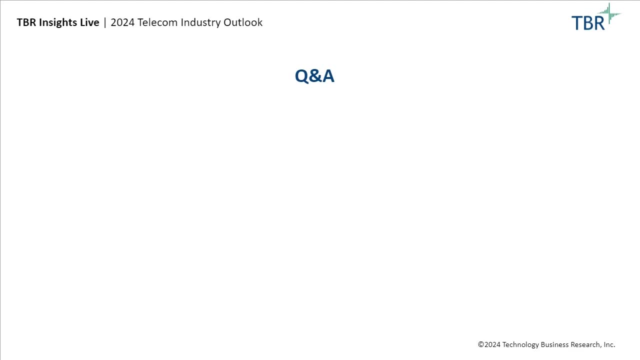 also impacts pricing in markets and that would also impact roi calculations. so i think, when you take all those things together, it's driving those um overarching decisions. so the next question is: which markets do you see m&a picking up? okay, so um india, something needs to happen with vodafone idea. they are. this is well known um and it has. 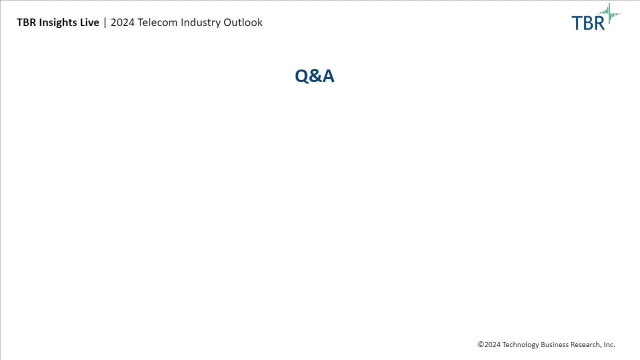 been well talked about in the industry that they have a financial crisis at that company and there needs to be a solution this year. they can't wait any longer. something big has to happen with that company this year that will either put them on a path to recovery or will redistribute those. 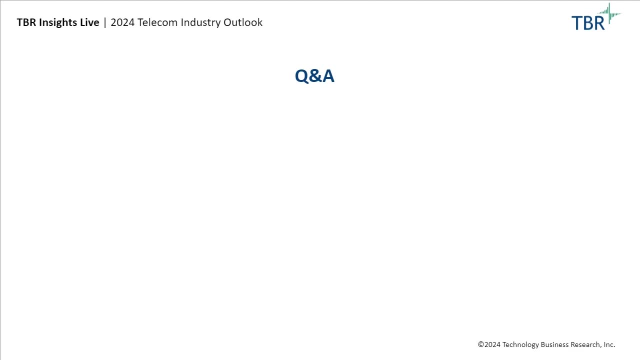 assets to other entities. um, so that would be one example. um, we would expect ma in europe, we expect mna in the states, we expect quite a bit of m and a in the states. actually, um, there are a lot of, are several companies. I'm not going to name names, but there's several companies that 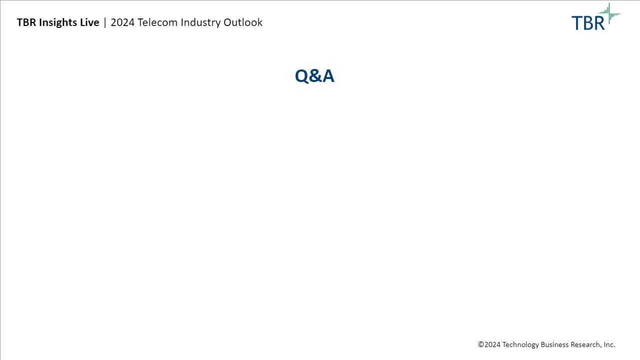 their finances have deteriorated to the point where there will need to be a significant change in their financial picture this year. They are not going to be able to push the can out to next year. It's going to have to be this year, And that could be Chapter 11, debt restructuring. 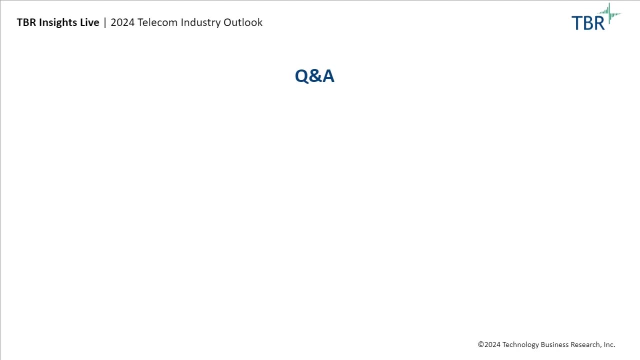 It could be Chapter 7, where there's a redistribution of assets to other entities. It could be a partial or full government nationalization. It could be an asset sale, So it could be a line of business. It could be certain assets. Maybe there's real estate that. 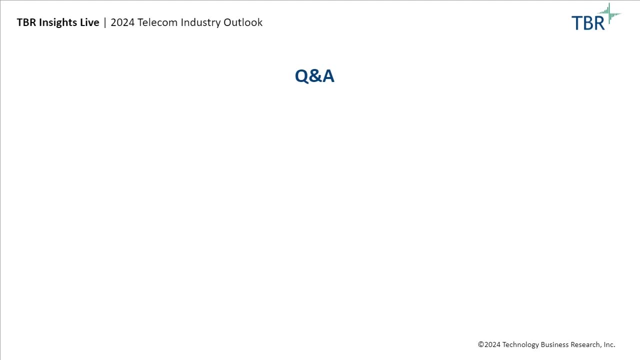 a company is carrying that they want to sell off. Maybe there's spectrum that a company has that they have determined to sell off. All of those types of situations would be in play, especially in the US market. Okay, Next question is: 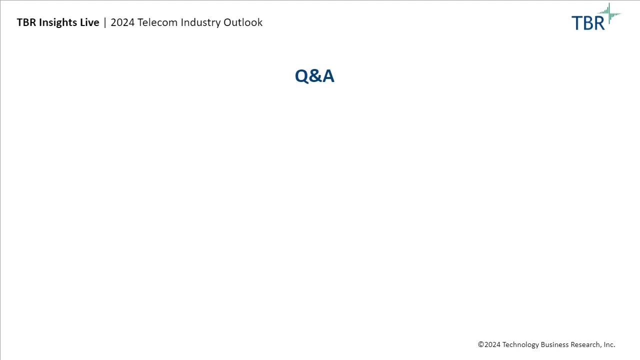 Yeah, So someone mentioned some other Another example of M&A. I'll just mention It's Orange Spain and MassMobile. So yes, thank you for mentioning that. That is another. That is another example underscoring that the M&A environment is heating up. 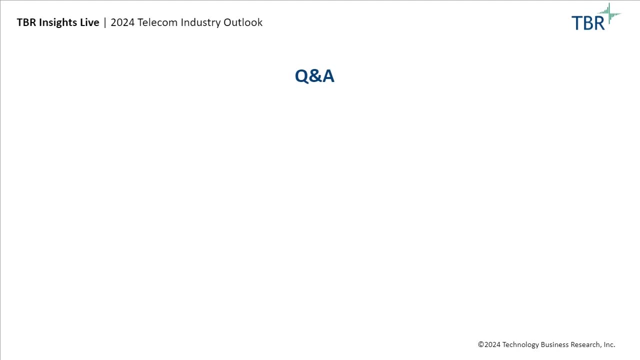 And again, these combinations now where the number one or number two player is buying the number four player. those are happening now. Before those things would not have been considered by regulators, So that's a change, All right. The next question is: who are the vendors in the cash flow predictions? 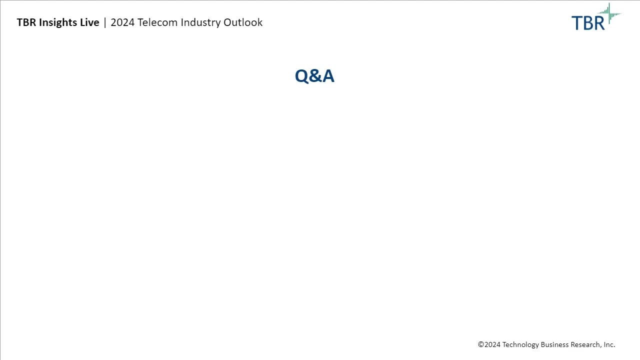 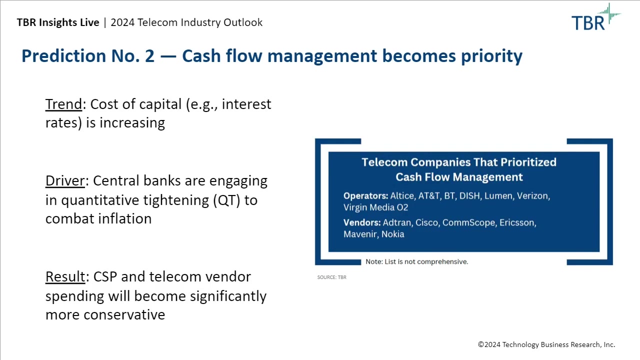 I missed the slide. All right, I'm going to go back that slide. I think it was this one. Yeah, So this is the list, Again this list, since we wrote this report in November of last year. since then, we would be adding more names to this list that have come out and explicitly said that they are. 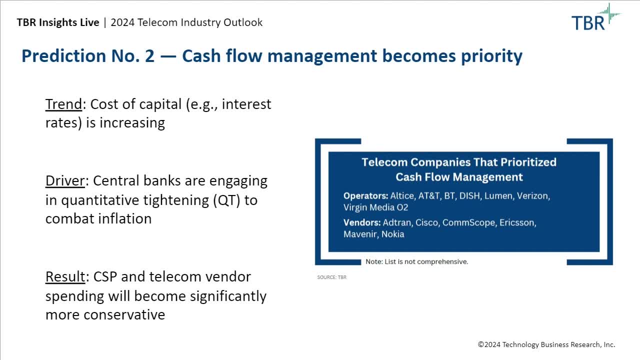 We are prioritizing cash flow management. Cash flow management is the phrase that we're using to wrap these into, but they will use different phrasing and words to describe this, but they're basically describing the same thing, So we're just wrapping it under the notion of cash flow management. 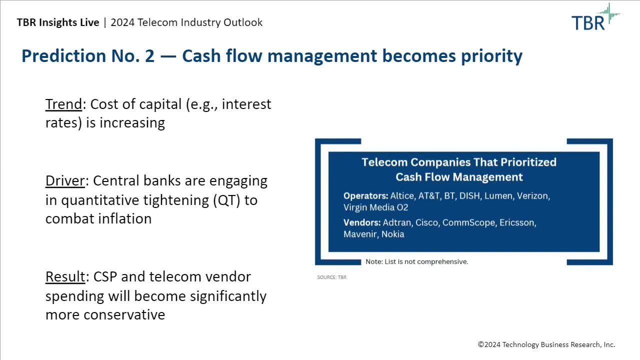 The next question is: when do you see ROI coming in for 5G investments? There's so much discussion on monetization and I still see operators struggling. So, yes, when, When, When, When, When, When, When. 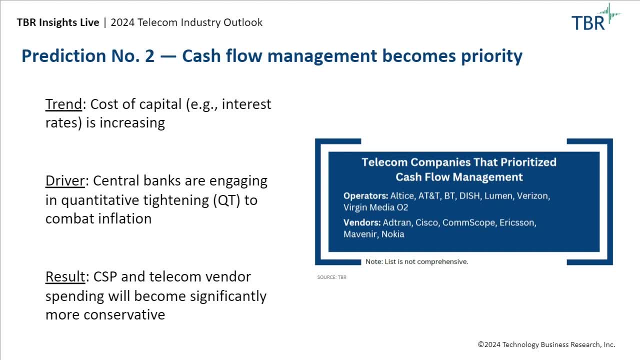 So, ultimately, I do believe that 5G will bring you know. 5G, in conjunction with AI and edge computing and those new technologies, because a lot of them interwork with each other to bring outcomes. Trillions of dollars in new economic value will come from these technologies, including 5G. 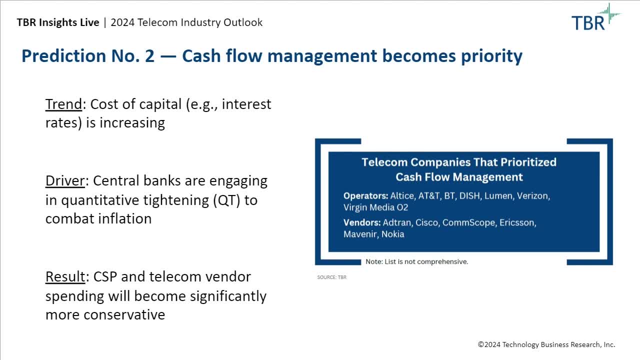 It is going to happen. I'd say we're at the very, very early stages of this. still, Even though we're five years into the 5G cycle, we're still at the very early phases, or early innings, if you will, of the actual monetization of new business models from that technology. 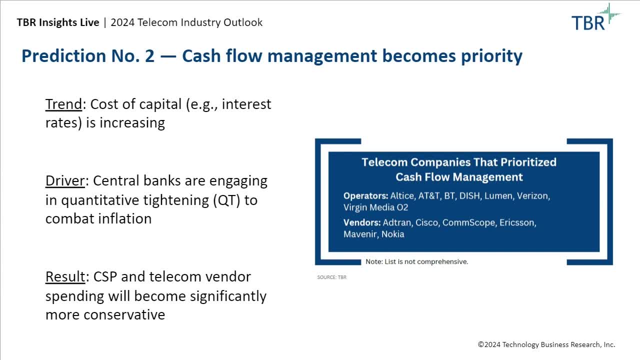 I think that we're going to see as this decade moves forward. I would expect in the later years of this decade we're going to see telcos generating significant new revenue from 5G. Okay, Okay, So there's still a ways to go. 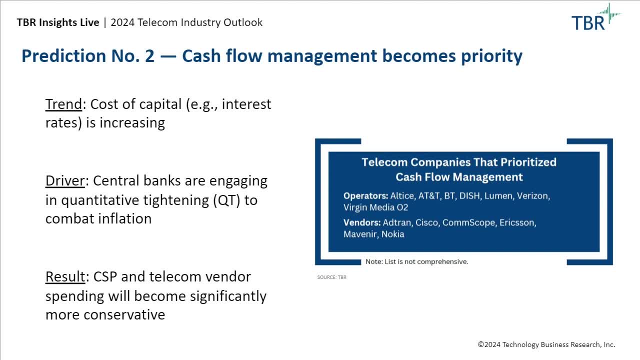 Again, I'm excluding FWA from that. Like other things beyond FWA, we're still a couple years away from scaled positive ROI. you know use cases that are driving a positive ROI for the telcos. Okay, The next question is any specific observations for 5G Open RAN rollouts in Europe. 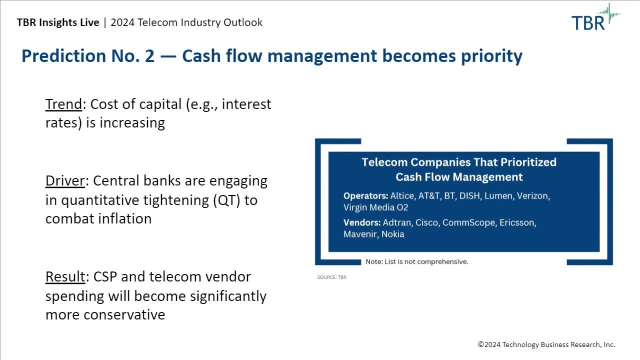 So Open RAN is still happening regardless, Despite the challenges, but the scope of what's happening is much smaller than people were originally expecting. The industry was originally expecting that there would be large-scale macro network deployments of Open RAN. What has wound up happening? maybe with the exception of DISH in the US and maybe Rakuten in Japan. 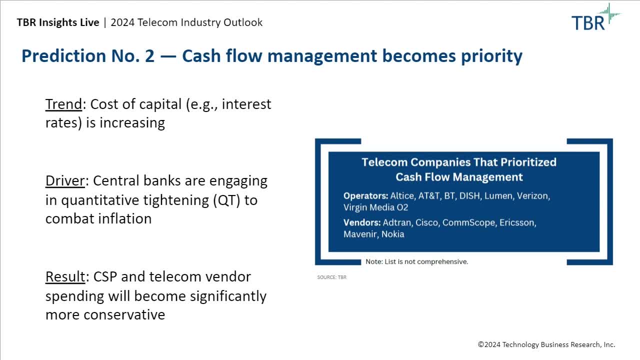 So maybe a couple telcos would be exceptions to this rule, But any telco with brownfield networks. what they have wound up doing with Open RAN is very small-scale trials pilots, or they're using them for a very specific use case, like small cells in building, as an example. 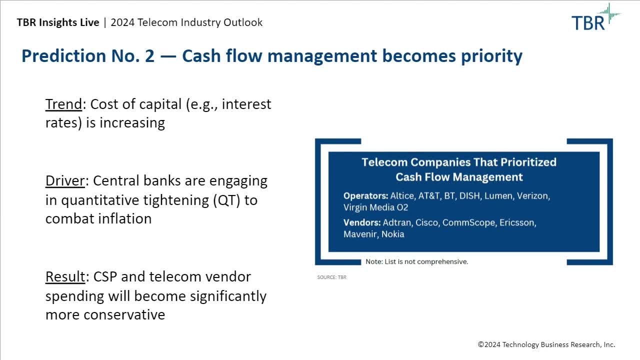 Introducing Open RAN into brownfield macro networks is not happening. It's not happening on a commercial level. Maybe on a pilot or trial level it is, But from a scaled From a commercial perspective it's not happening yet And we do not expect that this year that's going to happen for brownfield. 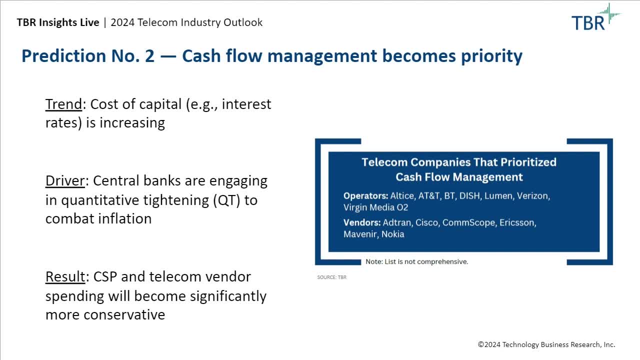 For greenfield it is happening For brownfield. we're not expecting a big catalyst this year. The next question is: are competition regulatory authorities prepared for the likely uptick in M&A, bearing in mind the BTE deal in the UK? 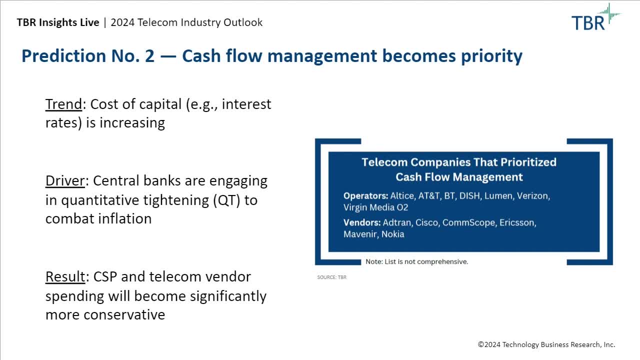 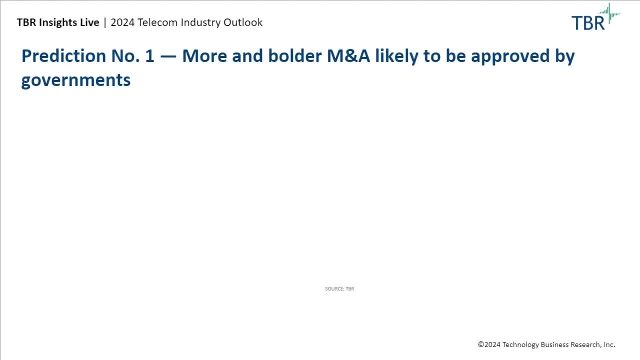 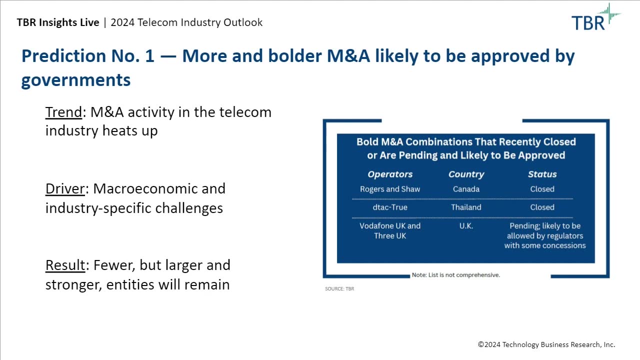 Sorry, If you look at the trends- and we gave examples, I'll actually go back to that slide. So, if you look at these deals, two of which have closed and two of which- one of which that other person mentioned on another question- these are all examples where tier ones are buying up tier two, or maybe even 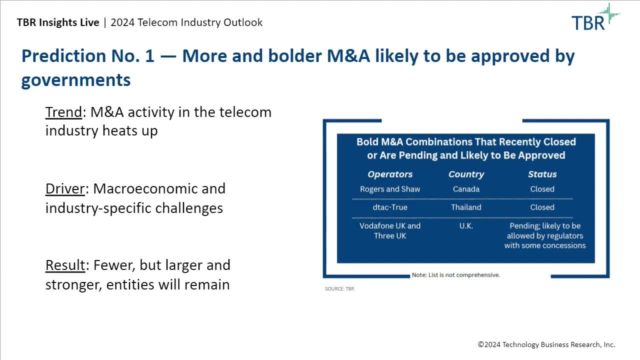 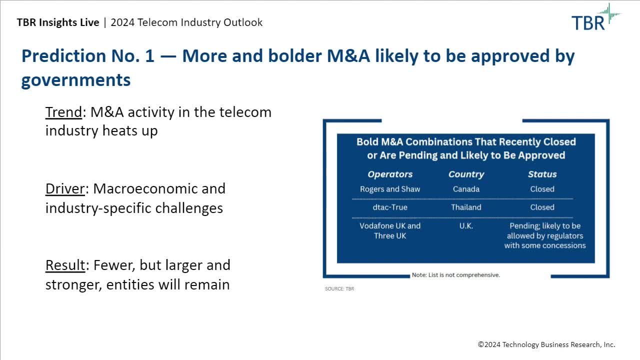 For all intents and purposes, they are being green-lighted with some concessions. So that is a change, And I do think we're going to see bolder M&A. We're going to see more tier ones come into the market with deals setting up, deals for horizontal M&A, and we may even see some vertical M&A. 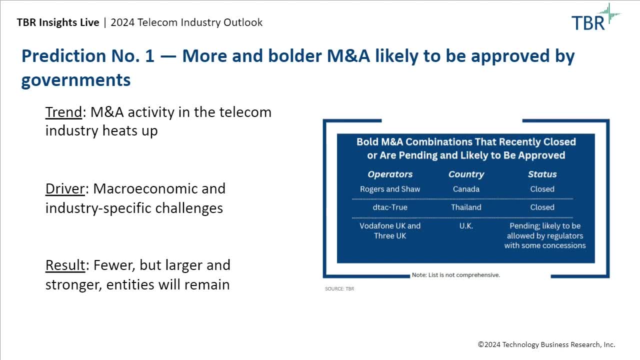 but we're expecting the majority of the M&A to be horizontal in nature. Remember, telco is a scale game on the vendor side and the operator side. They're going to be looking for situations where they can enhance the economies of scale so that they can offset. 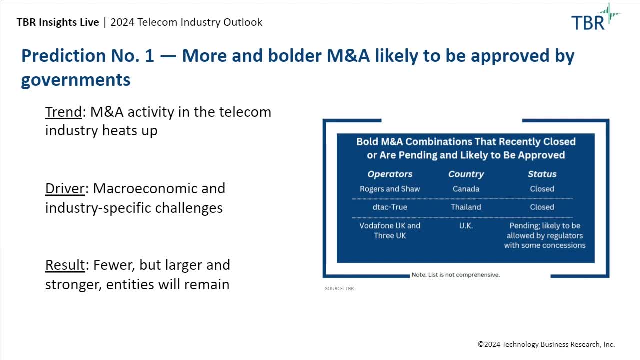 maybe revenue erosion or flattened revenue, and they can increase their earnings per share by getting that scale. So those are some of the things to keep in mind there. All right, the next question is: how do you see sustainability playing in the telecom industry? 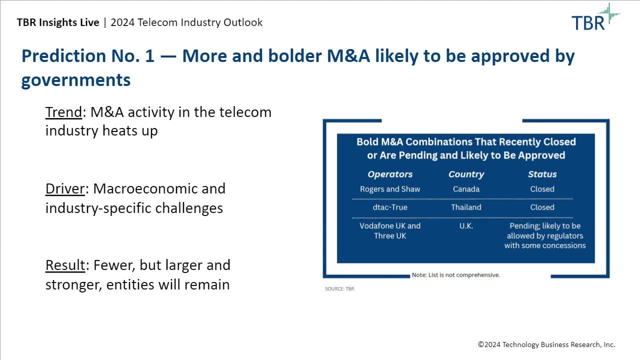 What are the key initiatives operators are embarking on for sustainability? So, from a sustainability perspective, the majority of what we see from a telco perspective is energy management. So anywhere where they can get energy efficiencies, that's where they're making investments. And I'll give 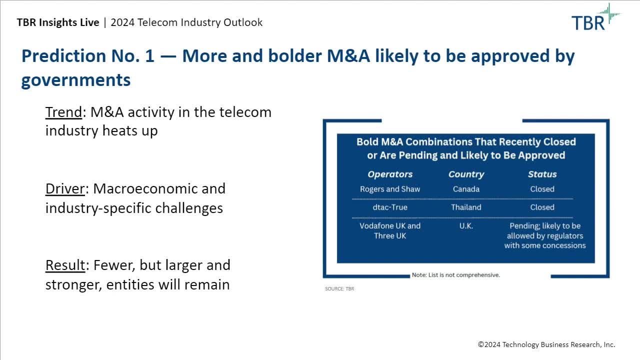 you some examples of this. I'm not going to name names, but there is a tier one vendor that has an energy SaaS solution that they sell to operators. They have a few customers in Europe. I'm not sure if I'm allowed to disclose them, so that's why I'm not mentioning names here. 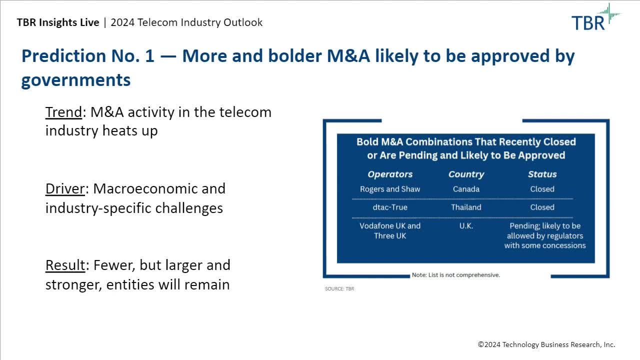 But they are running their radios on this platform and they have realized, I think, somewhere between 5% and 15% reduction in energy usage of that radio environment at scale. So if you think about energy costs from a telco perspective, that's one of the biggest.